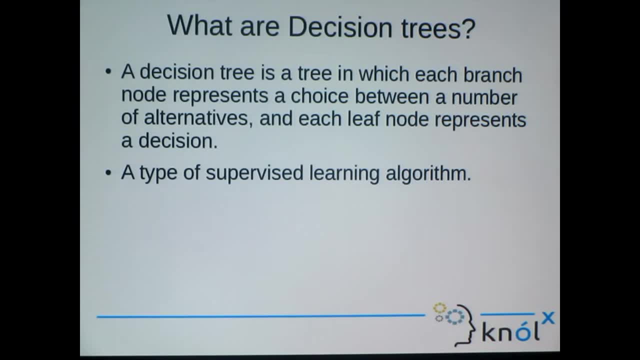 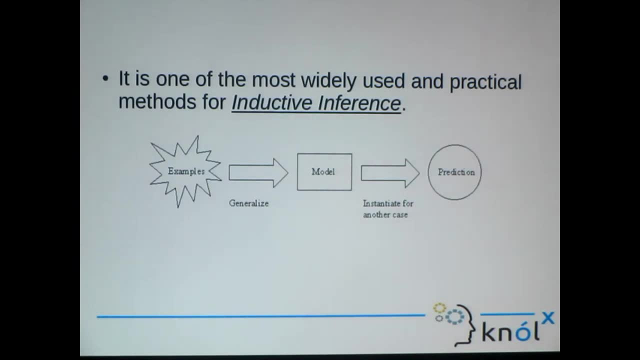 So decision tree is a type of supervised learning algorithm. It is one of the. it is one of the most widely used in practical methods or inductive inference. But what is inductive inference? It is a process of reaching to a generalized concept with the help of specific examples. 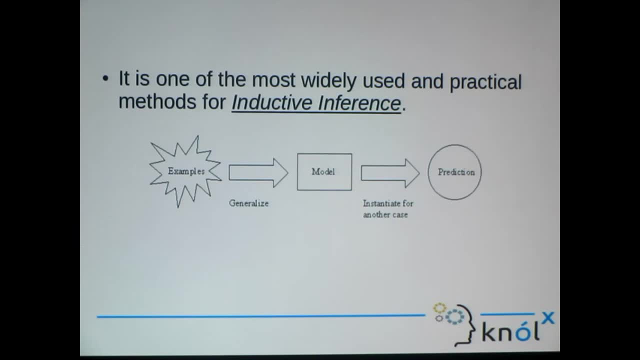 And decision tree is based on this. That means we are provided with the examples, specific examples, and we will conclude a generalized concept and with that concept- generalized concept- we are going to find the decisions for the unselected. We are going to find the decisions for the unseen- examples. 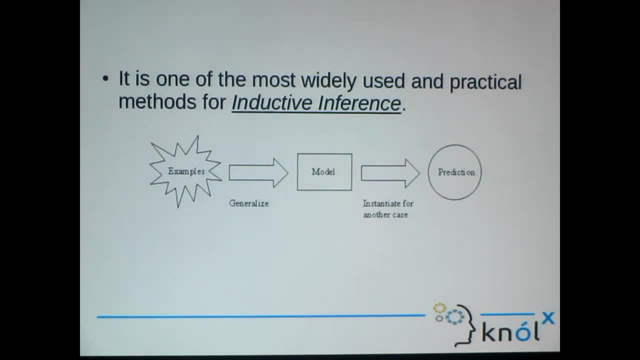 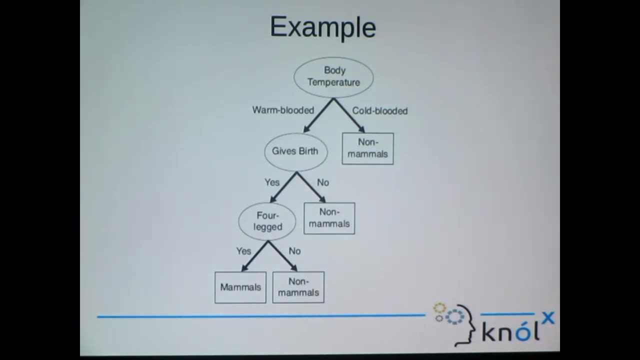 So this is the whole idea about general decision trees. So this is the graphical representation of a decision tree. It is very simple. Root node contains body temperature, where it can be either warm-blooded or cold-blooded. If it is cold-blooded, we say it is non-mammal. 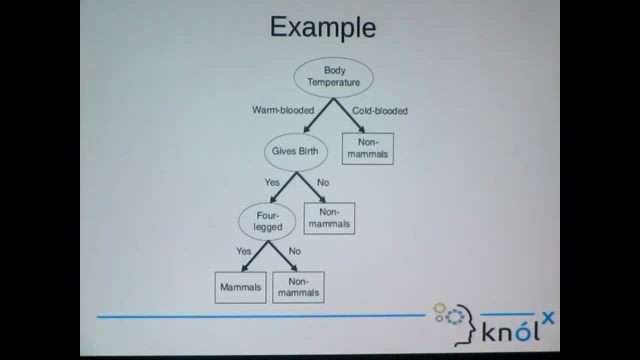 If warm-blooded, then we will check again whether it can give birth. If yes, then we will check again whether it has four legs, And if it has four legs, then we will categorize it as mammal, And if not, then non-mammal. 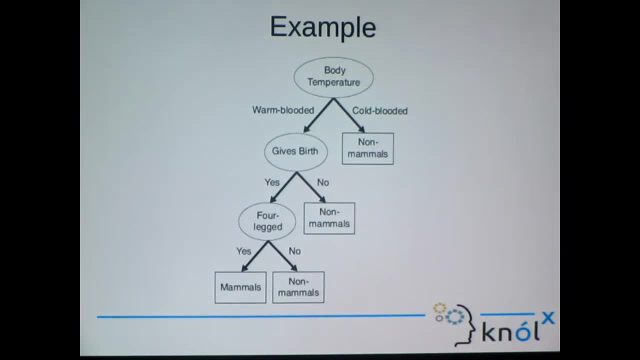 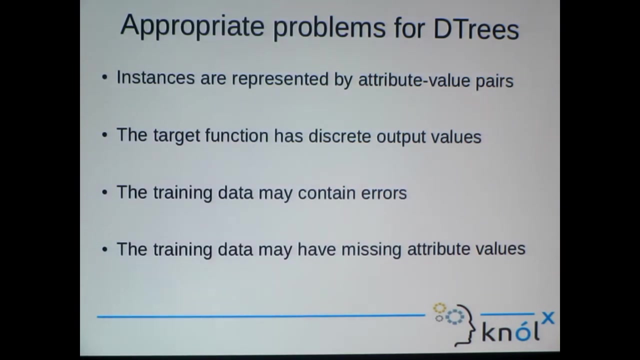 So, basically, we are trying to categorize things or examples to two categories, that is, mammals and non-mammals, with the help of a decision tree, And attributes would be given to us. So this is the decision tree. Now, what are the appropriate problems or the situations where decision trees are most appropriate to use? 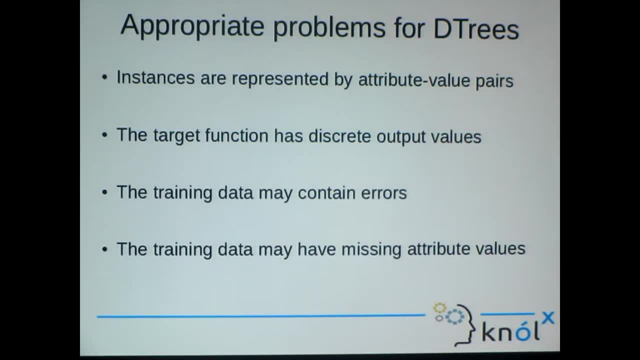 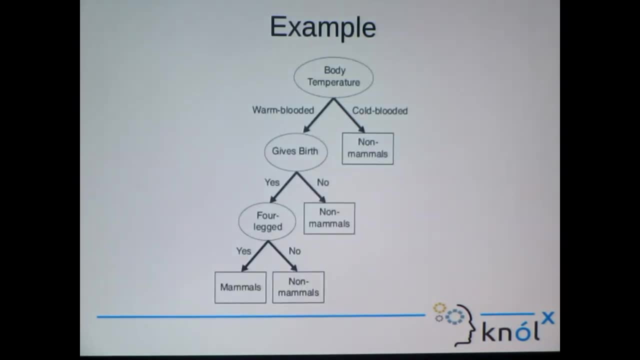 When the data or the instances are represented by attribute value pairs, like we have in the previous example. we know that body temperature could be either warm-blooded or cold-blooded, So there is an attribute and its values. So decision trees are most usable for in that particular situation, when we have attribute value pairs. 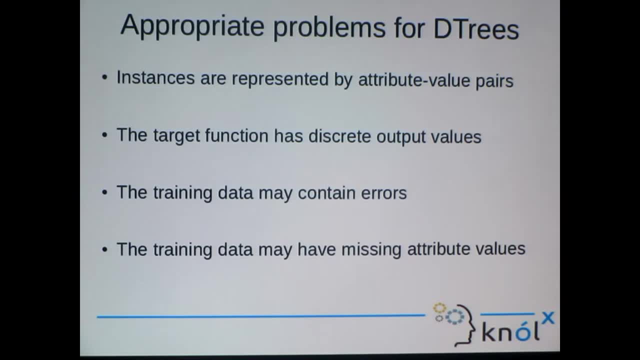 Second, the target function has discrete output values. That means the decision tree method would give the output as yes or no for classifying things. Training data may contain errors. That means decision trees are robust to errors. Errors could be like while defining, while categorizing the examples. 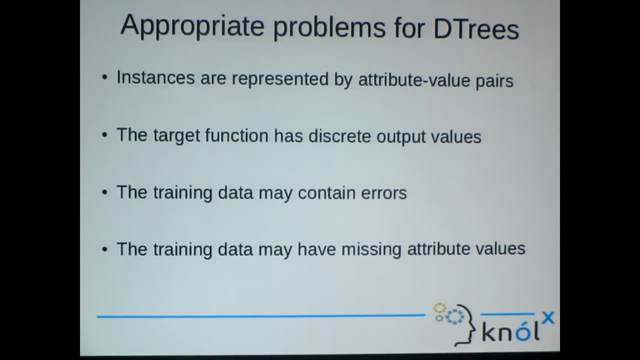 Or the attribute values can also have errors, So we can use decision trees in that case also. Decision trees can be used when training data may have missing attribute values. For example, I don't have values for whether it has four legs or not. 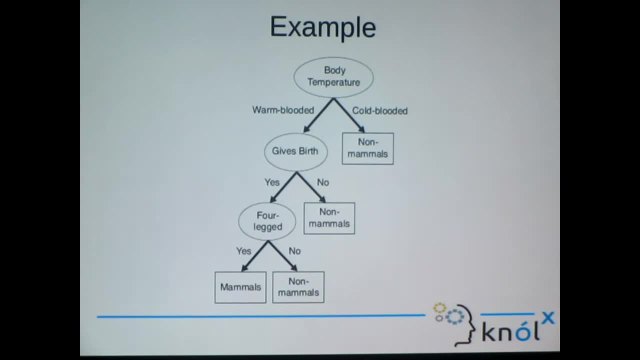 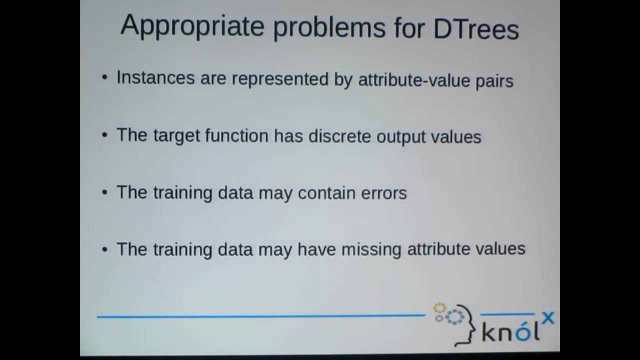 For some of the examples, I don't have this value, Even though we can use decision trees. Decision trees are used for the following reasons: Mostly everywhere, like in agriculture, astronomy, medicines, Like, if I want to classify the patients having serious tumour or having minimal one. 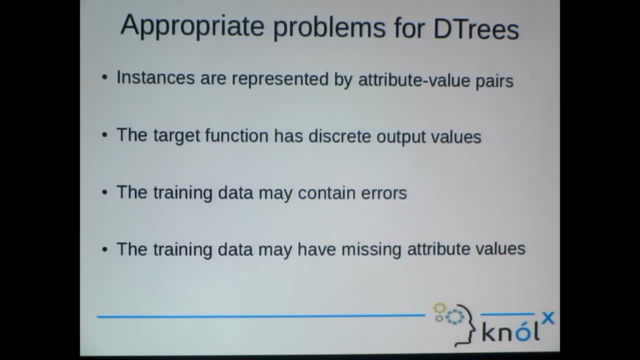 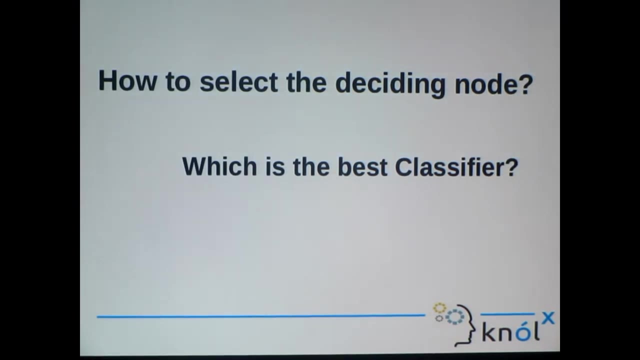 Or medicines where we can. patients can be categorized into different, different problems. So so far, so good. Like we have the problem, We make the tree, We get the tree, We get the decisions. Is it so simple? No, How do we get to know? 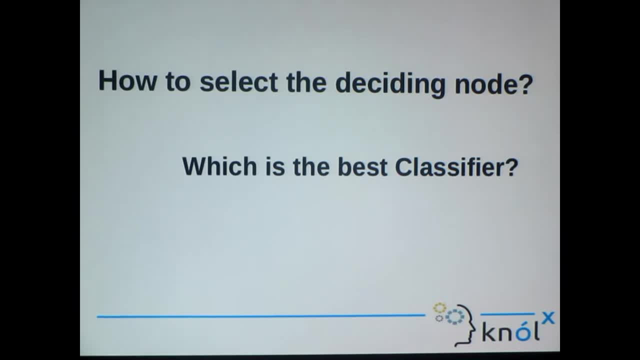 That out of all the list of the attribute values, which attribute is to select for the root node? We cannot just pick any attribute and put it as my root node. It will definitely gonna lead to a decision tree that would not help me in taking decisions correctly. 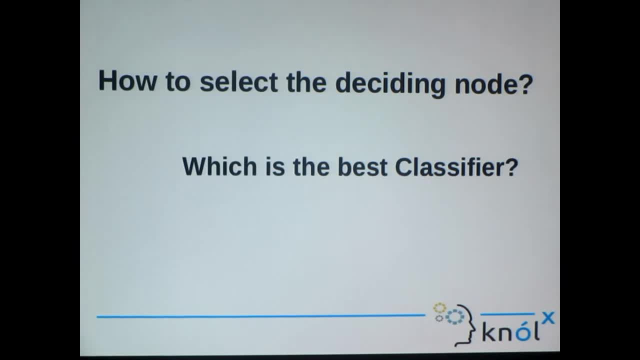 So there has to be a formula or some way out to decide which node to select, Which attribute to select As a decision root node, Before beginning. these are the. suppose these are the situations like A, B, C and which node can be easily described. 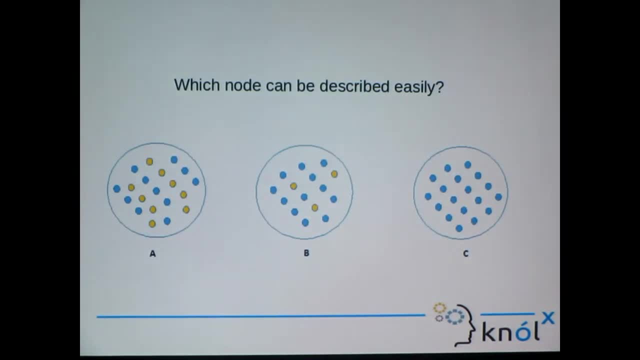 Of course the answer is C because it contains all the blue balls, So I don't need any much information or anything to you know to conclude this, That I don't need much information to describe this one, Whether in B some are few are yellow and most of them blue. 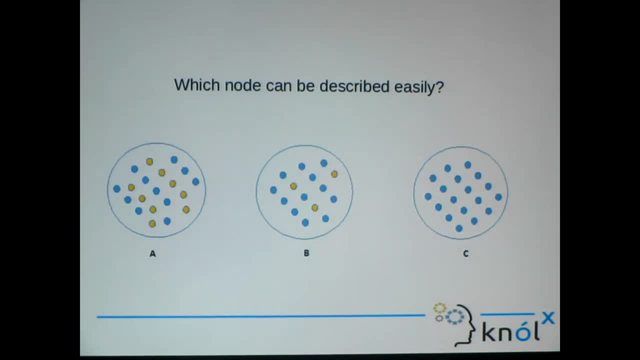 So I don't. I need information, but not that much. I will be able to classify this one, But in case of A, in which yellow and blue balls are randomly categorized, This organization is there. So I need more information in case of A and less information in in C. 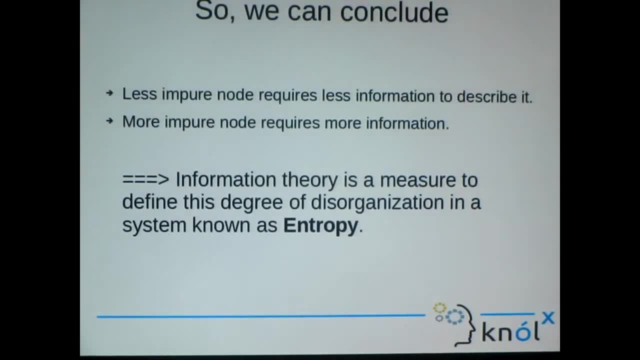 So I can conclude that less impure nodes, Less impure node requires less information to describe it. If it is impure, less impure, Then I don't need any information. I will just classify it, It will be no problem. 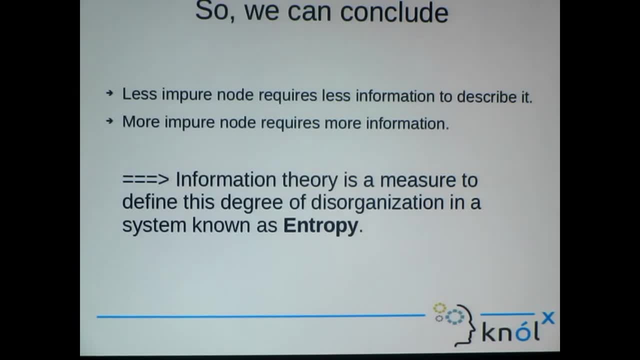 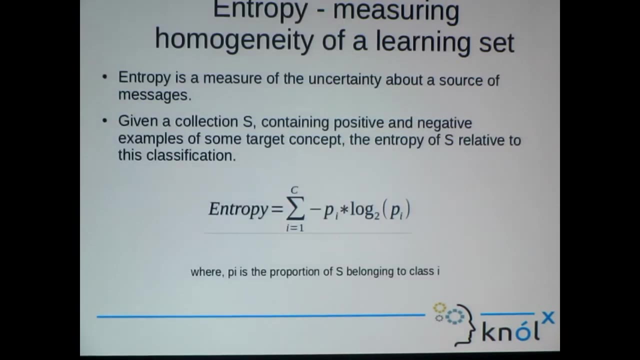 But if it is more impure, I require more information to classify or to categorize that node. So this degree of disorganization in a system is called entropy. This is the exact definition that does entropy. Entropy is the decision of the uncertainty about the source of messages. 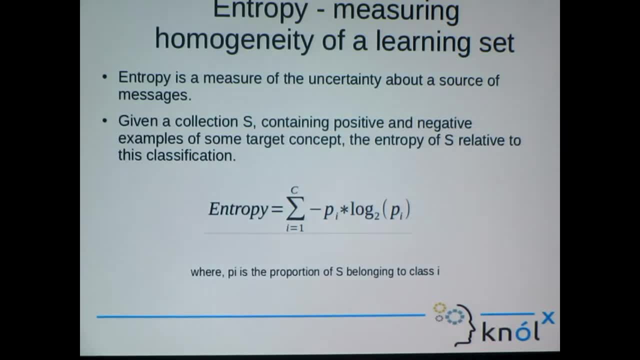 I have data, I have a collection of data And some of have impure data. right Data is disorganized, So I have to. there has to be a way that I can categorize this data, And entropy will help me in gaining that information. how I can categorize that. 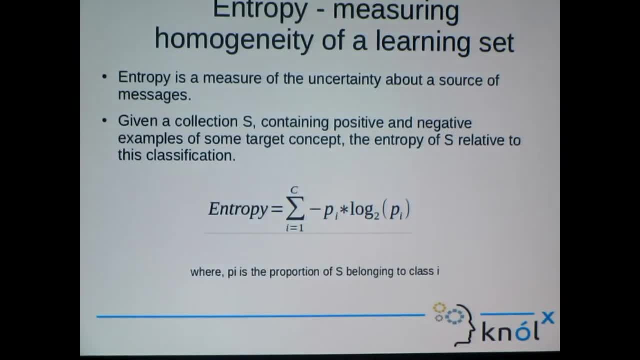 So this is the formula for calculating entropy In this, where P is the proportion of proportion in S Like. if I talk about positive ones examples, Then how many positive examples in the data set are there? So I will calculate entropy with this formula. 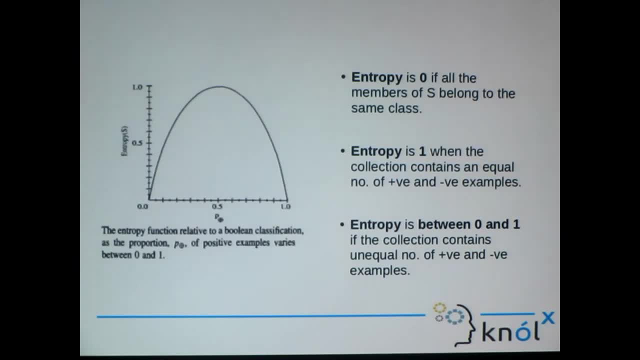 Let's just explore more about entropy. This is the graph of entropy function versus P. positive examples. Suppose I have a collection. There are positive examples and negative examples, right, And this is the graph When I will have P positive. I am talking about positive examples. 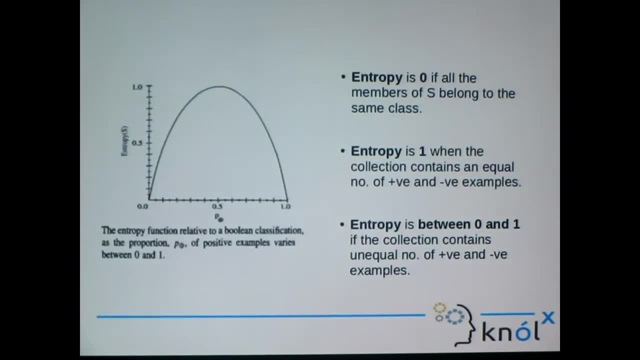 If I have zero positive examples, that means I have only negative examples in the set in the collection. That means my entropy is zero because there is no impurity. I don't need anything, any information, to classify those things As I move forward towards along the x axis. that is positive examples. 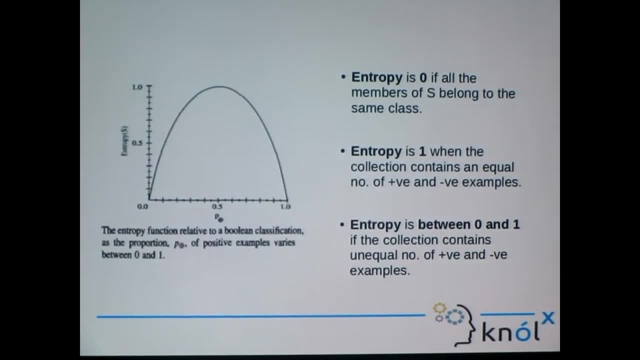 my entropy will increase. That means I have now I have a negative examples And positive examples, And when I reach in the middle that is 0.5, that means half positive and half negative examples- Then my impurity will be the highest one. 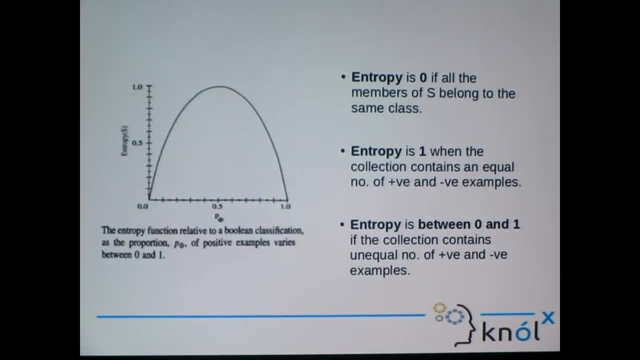 Then I need to organize that data. I need more information And as I move towards 1, that means I have more positive examples and less of negative examples, So my entropy will again decrease. So entropy is zero If all the members of S belong to the same class. 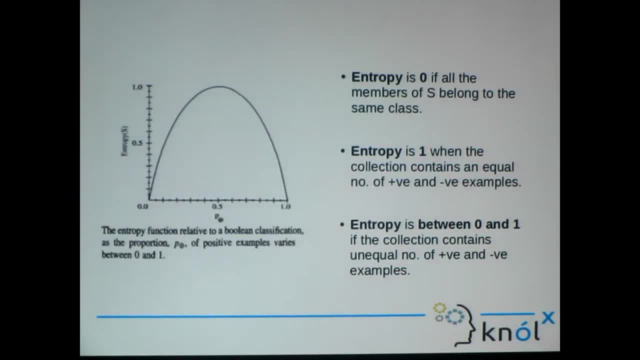 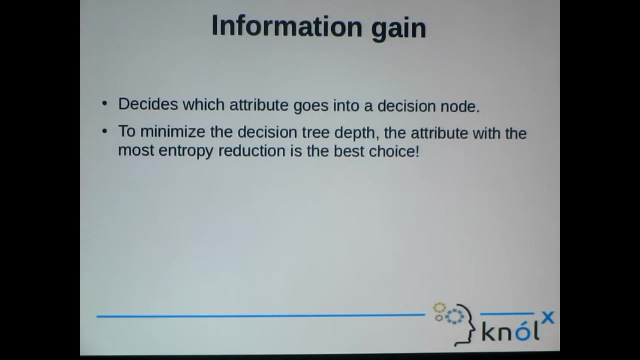 Right Entropy is one when we have equal number of positive and negative examples, And it is between zero and one if the example contains unequal number of positive and negative examples. So this is the thing that is going to help me in finding which attributes to be put in the root node. 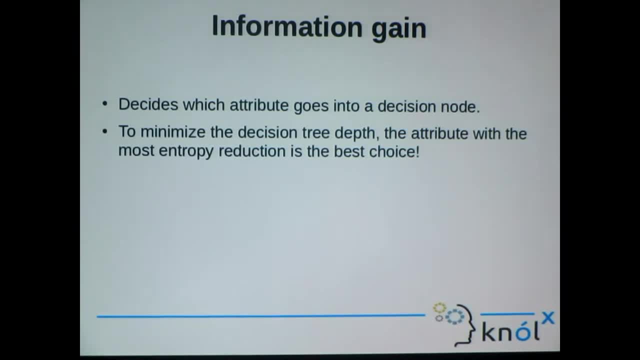 That is information gain. As the name suggests, how much information I can get from an attribute decides which attribute goes into the decision node. To minimize the decision tree depth, the attribute with the most entropy reduction is the best choice. Obviously, which attribute will have the less entropy. 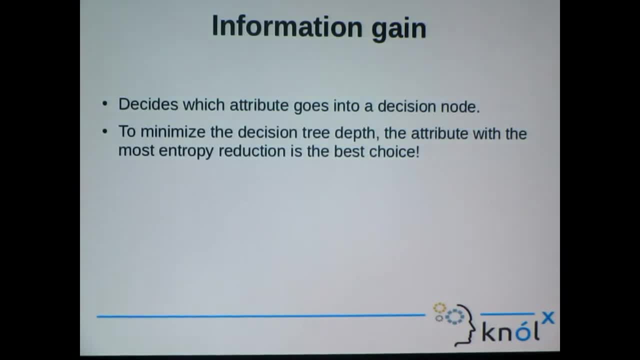 It will be my best choice. One thing I want to add: that taking an attribute without thinking of this entropy and information gain, I will put any node or any attribute over there And I will end up with the wrong decision tree. So I need to find information gain for all the attributes. 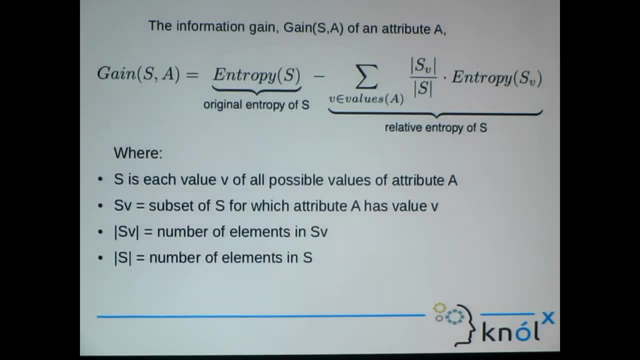 And this is the formula. This is quite big formula but it is not that difficult. Original entropy of S, that is, the collection of whole collection entropy minus the relative entropy of S. So we are going to find, suppose there are many attributes. 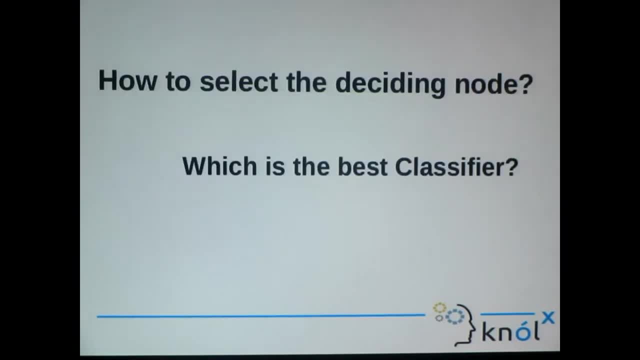 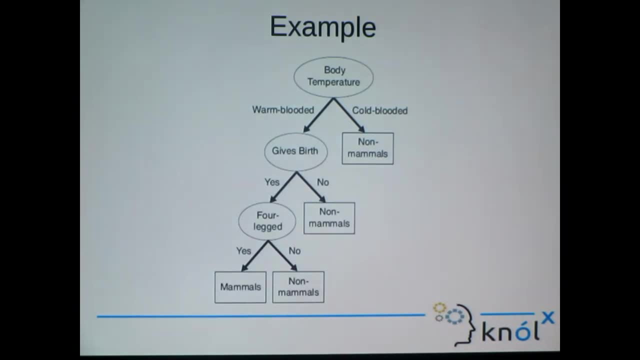 formula, like in the first example we have seen. we are going to find information- gain for body temperature gives birth, folded all the attributes- And we are going to find the values, whichever value is the highest one. We are going to put that as my root node. 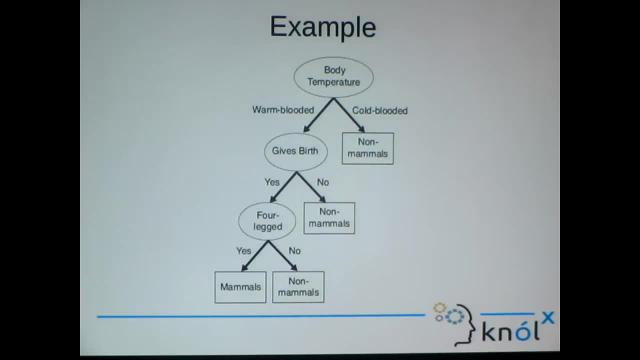 Because that is the attribute which is going to give me more information. What do you mean by highest one? Sorry, sir, What do you mean by highest one? Highest, whichever attribute will give me more information, gain value. That means it is the best choice. 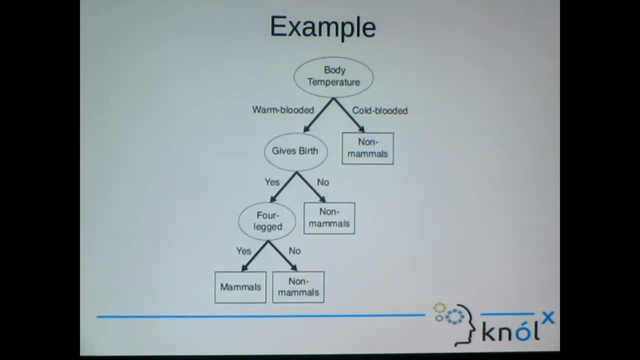 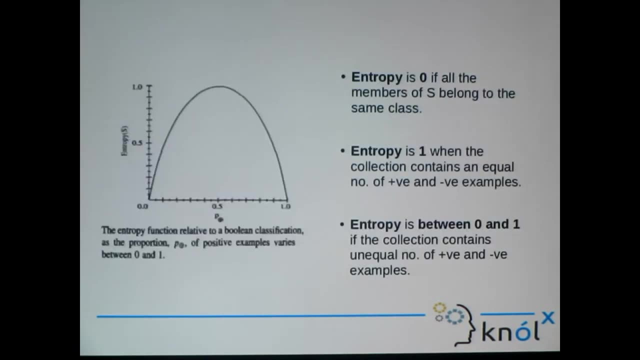 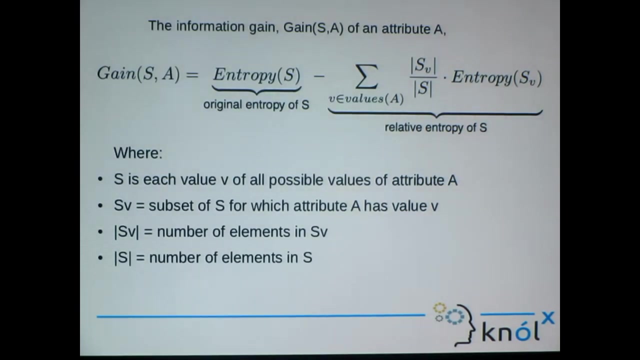 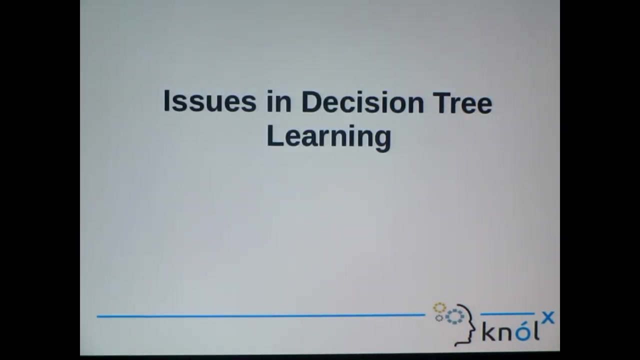 It will be helpful in defining the nodes particularly. We can see in further slides how it can help us. So that is information gain. So till now, we have selected the nodes, we have made the tree, everything is fine. Now we are going to talk about the issues in decision tree learning. 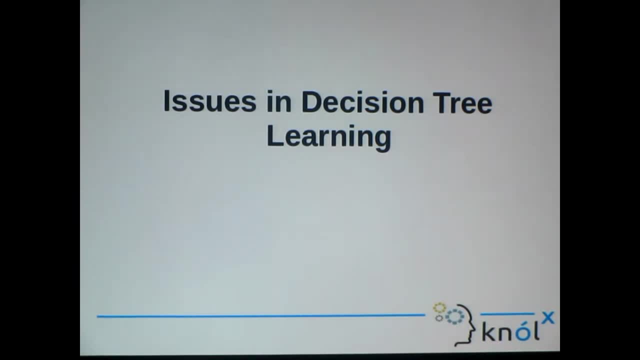 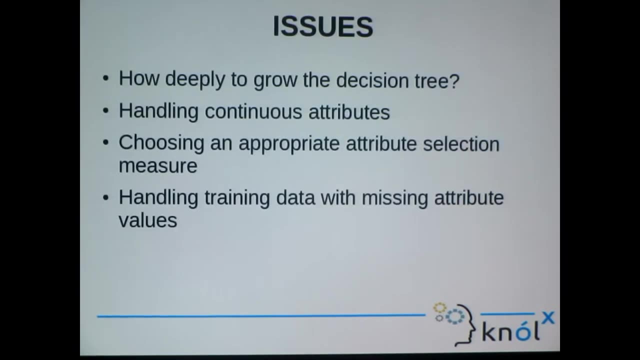 What can be the issues in decision tree learning? One thing we can think of: okay, the decision tree is not going to give me the best answer, Or the accuracy is not good. So these are the issues: How deeply to grow decision tree? 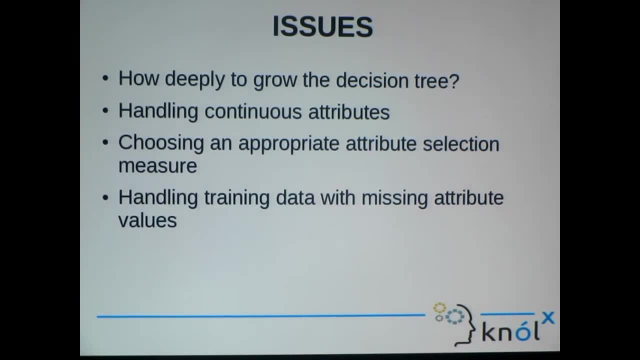 I mean we cannot just go. we have the example, we are just not going to grow the tree Like. this is not the good approach. Handling continuous attributes: choosing an appropriate attribute selection measure, handling training data with missing attribute values: I am going to discuss only the first one. 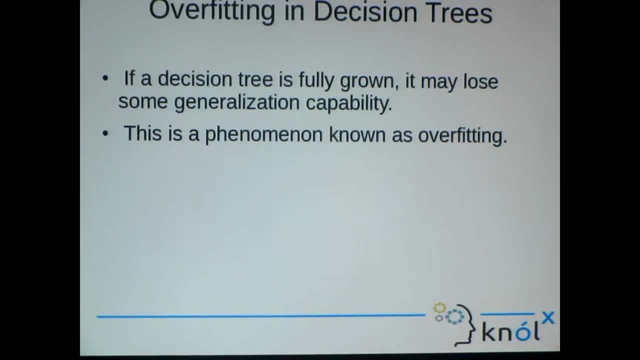 first issue: Okay, We have a lot of data with us to train my decision tree Right And, as per the example, I am going to draw my decision tree And, to fit that example, I am going to modify the decision tree. 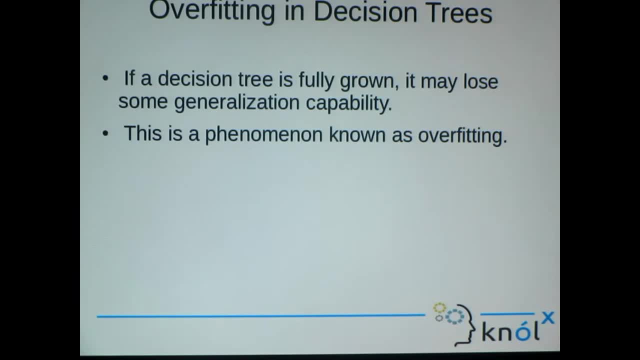 But now I have fit all the examples in the tree, But it will lose its generalization capability. This is called overfitting, Then that is, I am overfitting my data to decision tree without thinking about the generalization capability. Like this is the definition for that. 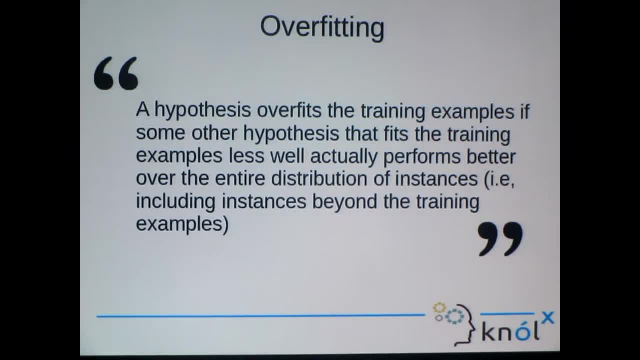 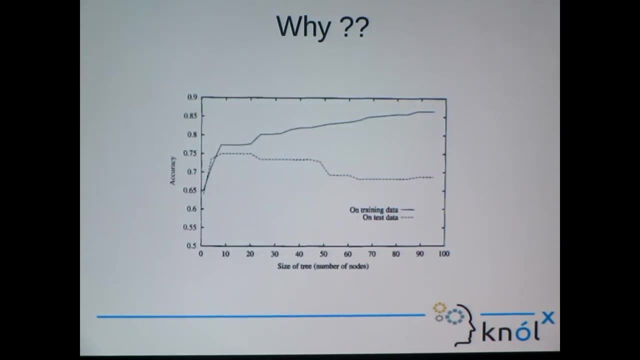 Hypothesis over fits the training example. If some of the hypothesis that fits the training example less well actually performs better over the entire decision instances, This will get clear with this graph more. Okay, I have made my tree. Now we have plot the data graph for accuracy versus size of tree. 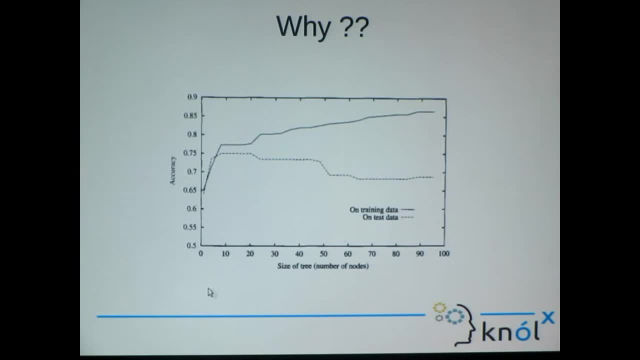 So, as you can see, I have made the tree with all the training examples I have And my accuracy is highest Because I have made all the examples, So it will be definitely going to be accurate for all the training examples. It will not give any error. 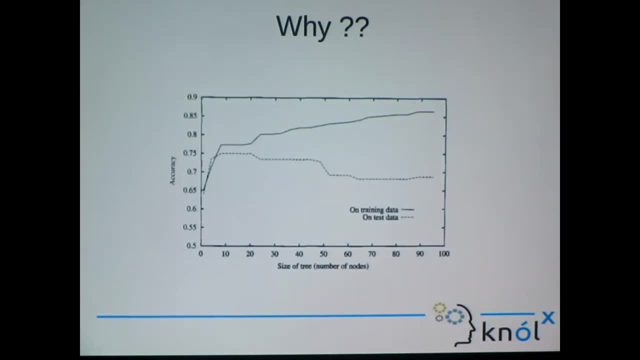 Because I have made the tree from that examples, So my accuracy will be highest. And then now I test this decision tree with the test data. With some other data that I have not seen, The accuracy falls. That means this accuracy does not match with the accuracy of the training examples. 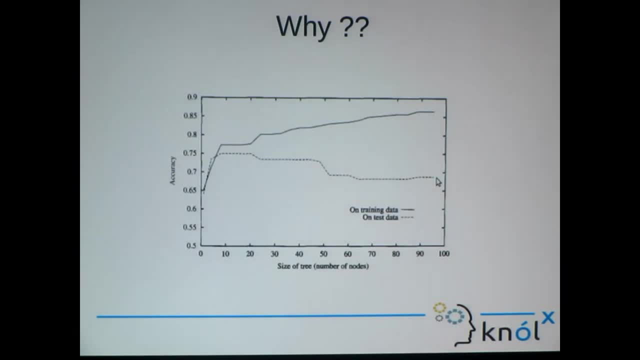 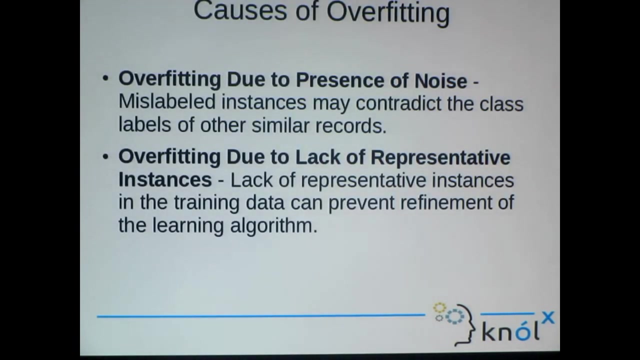 Why so? Because I- this is the reason- overfitting- I have overfitted the data. Hypothesis did not match Hypothesis data of the training, without thinking about the generalization capability. So what are the causes of overfitting? 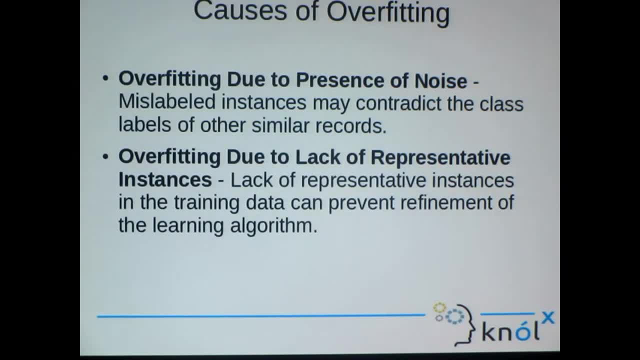 These are two problem causes: Overfitting due to presence of noise. That means my data is not correct, My data, we have some wrong or mislabeled data And I have blindly put it into my decision tree Just because I have to make that. 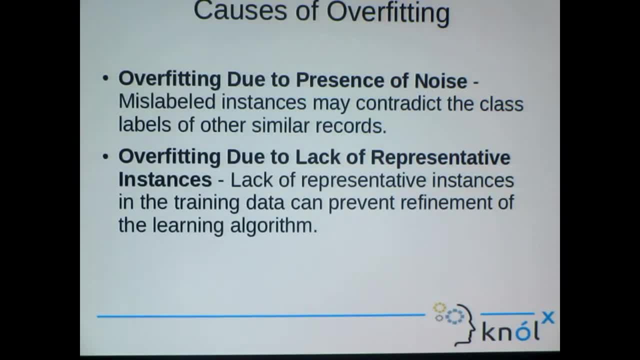 And second reason could be overfitting due to lack of representative instances. That means I don't have much of instances to put it in my decision tree, So that is going to end up in wrong decision tree, also Because I don't have much training data. 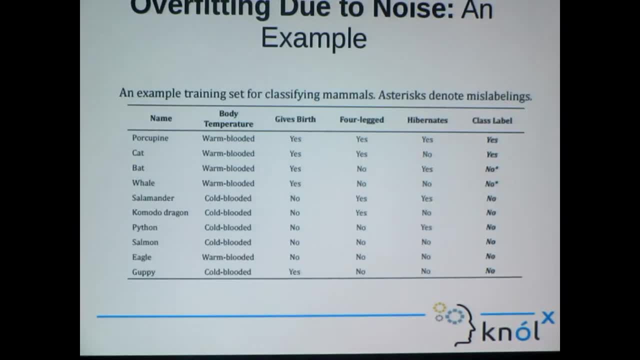 Now we are going to discuss each of these with the examples. See, this is the example for overfitting due to noise. That means I don't have correct data. The attributes are body temperature gives birth, cold, length, hibernates and the class label that I am going to give. 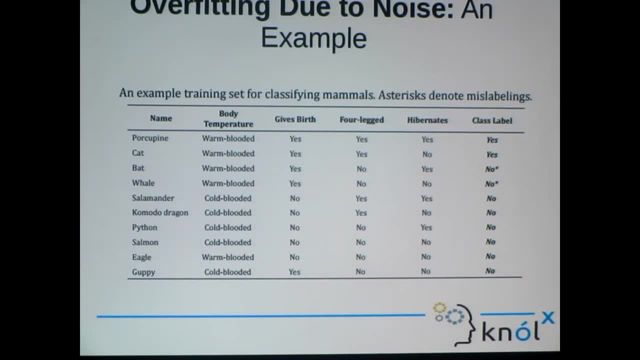 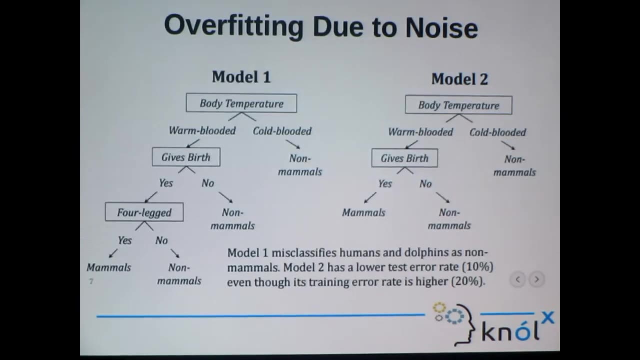 And my two of my data set is wrong. Asterisk denotes mislabeled, So two records are mislabeled. This is the data I am given with Now, if I make the decision tree out of it, I will make this one. 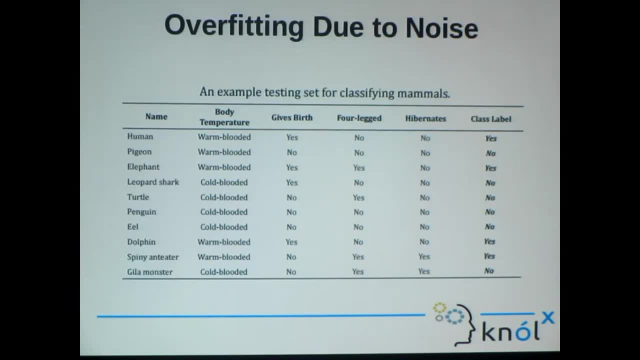 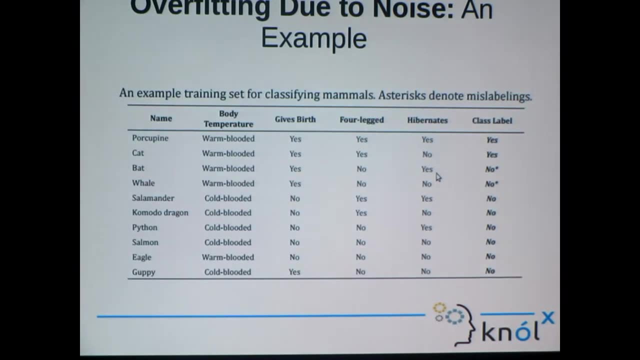 Right Body temperature, Then I will check upon. gives birth and cold length. This tree is made with this data. Decision tree will learn this data, apply it and make a tree, And the tree will serve this one only, This data set only. 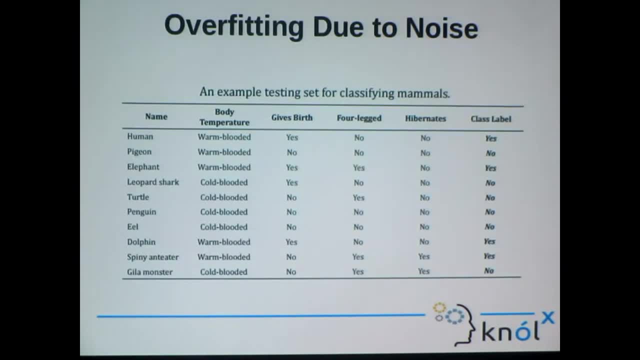 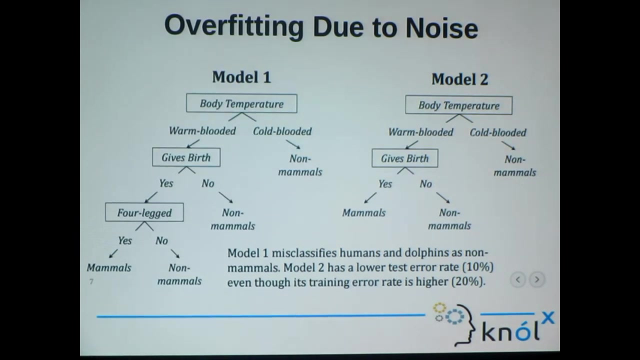 So, and this is my testing data- Now, if I check my decision tree, which I made through my training example, This is going to fail. Why? Because I have just told you that we just overfitted the training examples to get my decision tree. 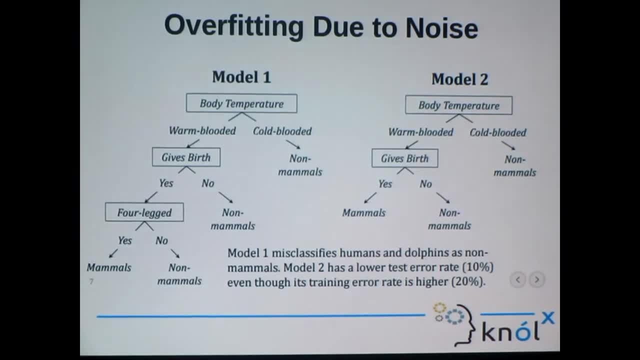 Like according to model 1, as sorry, model 1 will misclassify humans and dolphins as non mammals Because when it comes to body temperature, it will say: okay, warm blooded, Then gives birth, Okay, yes. 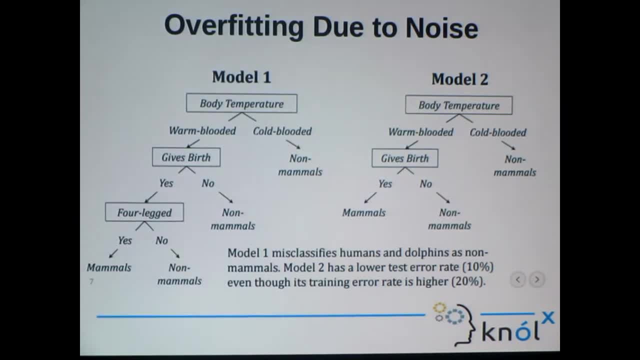 Cold length? If yes, only then. it is a mammal. No, Humans does not have cold length, So it misclassified it. So my decision tree is wrong, Because I have made this decision tree according to this data. 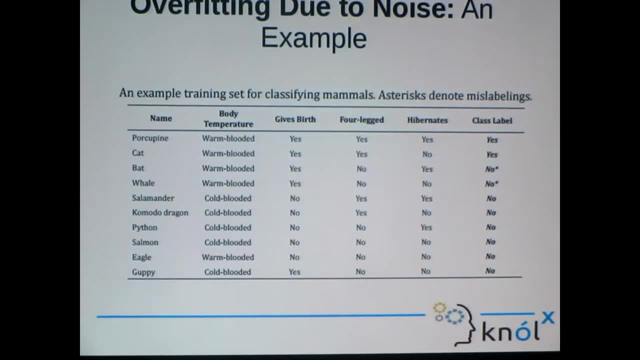 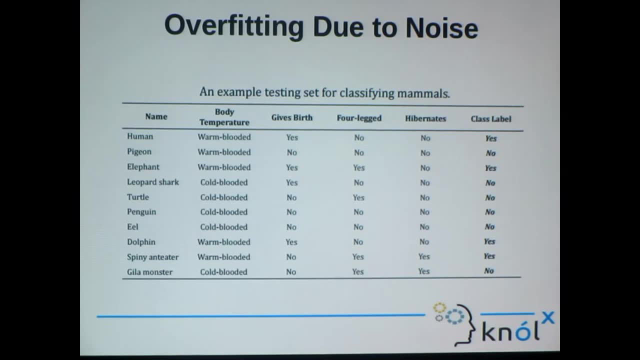 which is already impure or mislabeled. So I end up with the wrong decision tree. So the conclusion is: I would have to overfit the data Right And model 2 is made with the with this data. 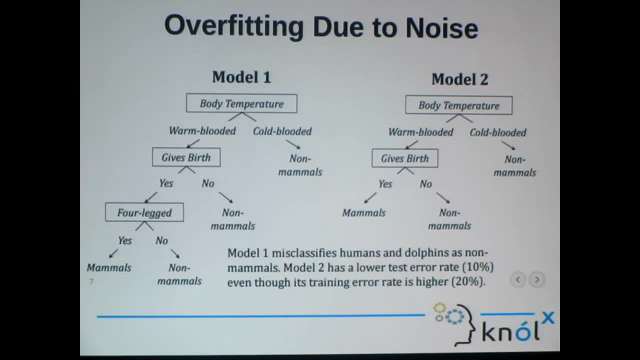 So when I check this one, that means the difference between model 1 and model 2 is this: that it does not have cold length attribute with it, So model 2 will fit that thing. Model 2 has lower test error rate. 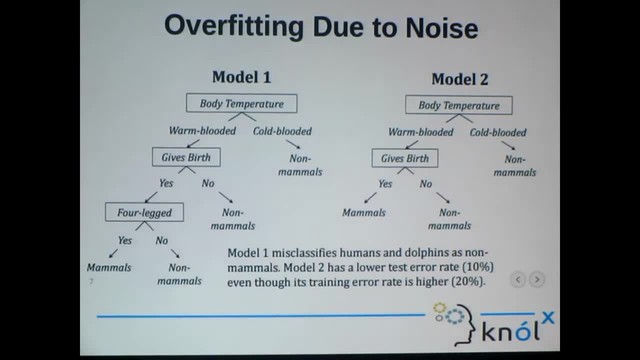 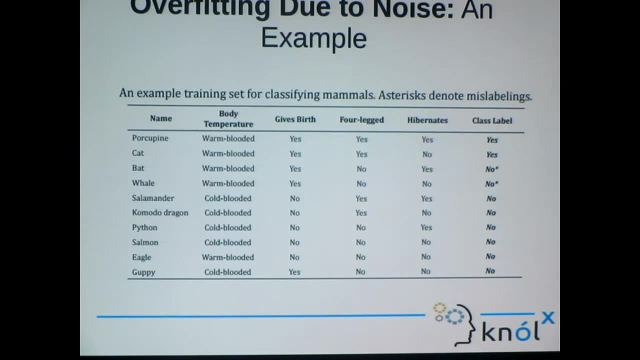 that is 10%, Even though its training error rate is higher, 20%. Okay, what is this error rate is when I- these are the two attribute records which are mislabeled. So 20% would be my training error rate. 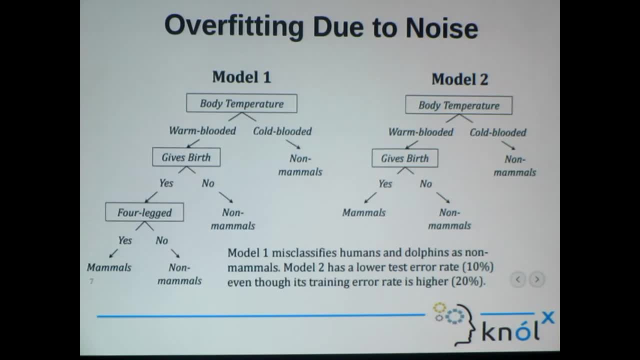 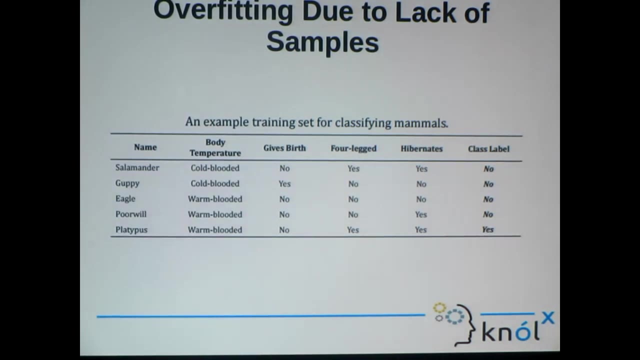 So the whole conclusion is this: that I am not going to overfit the training example blindly. I need to see which are what I am actually adding to my decision trees. Second cause is that, due to lack of samples, I do not have much of the examples. 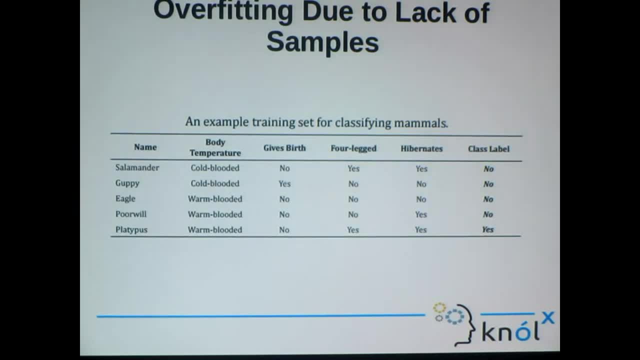 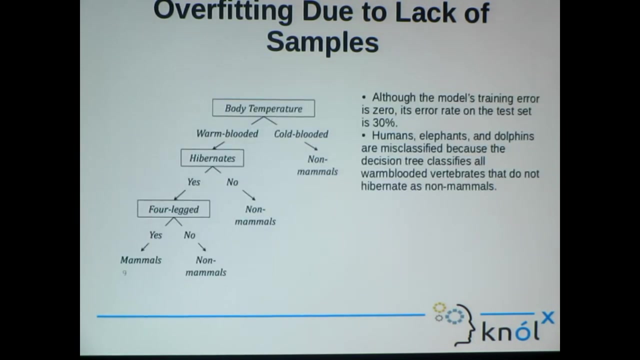 I do not have enough training, enough training samples to make my decision tree. That will also cause a wrong decision tree. So, according to this data which says if cold blooded and gives no birth has cold legs, it is not a mammoth. 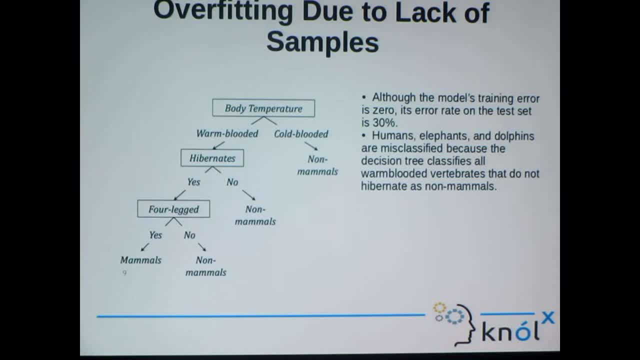 So according to this model, training error is 0. Why? Because I made this tree because of the training data only, So it will give 0 error. But when I check this in my test data it will give 30% error. 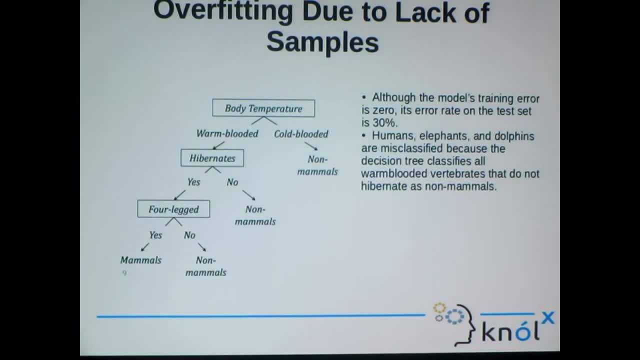 Wrong classification would be done, So as it will classify humans, elephants and dolphins- misclassified, as it says, warm blooded vertebrates that do not hibernate- as non-mammoths. So we have seen that, due to lack of enough examples, 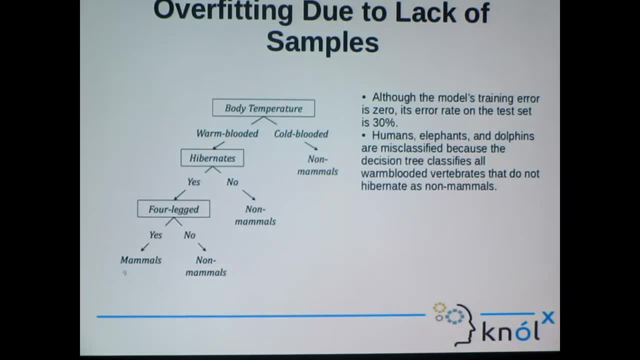 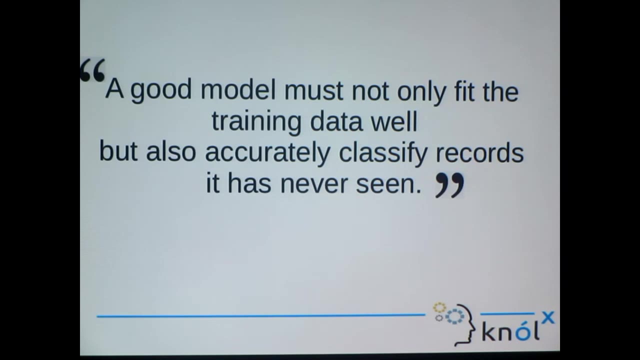 and, due to impure data or misclassified data, will end up as a wrong decision tree. These are the causes. So a good model must not only fit the training data well, but also accurately classify records, as it has never seen, And this is not just with decision trees. 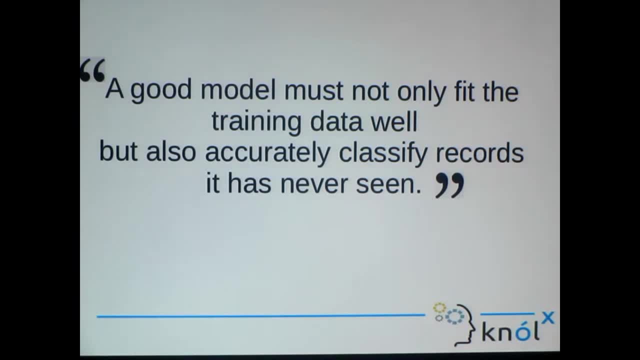 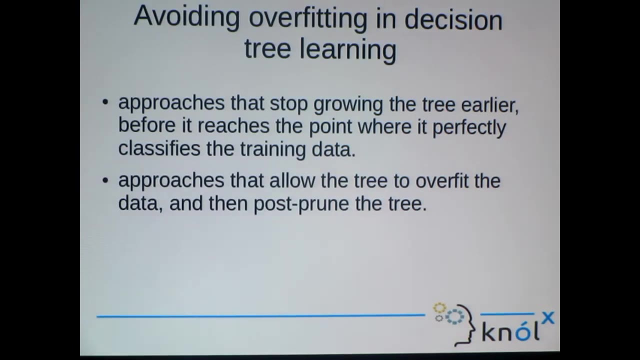 It is with every machine learning algorithm. We are not just going to blindly over fit the data, as it will end up in the wrong machine learning algorithm. So how to avoid over fitting, There are two approaches to that. First is stop growing the tree earlier. 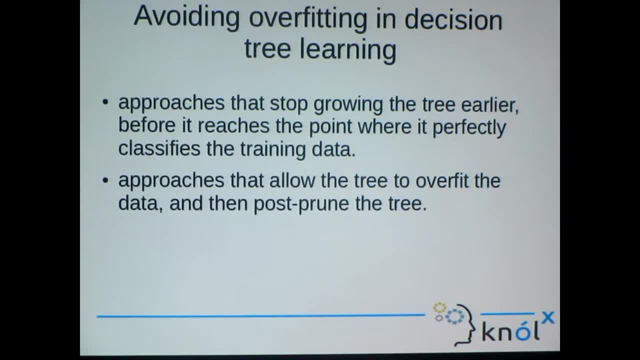 before it reaches the point where it perfectly classifies the training data. I am not going to fit all the data. I am going to halt the growth in between. only Second approach is let the tree grow over, fit all the data and post prune that tree. 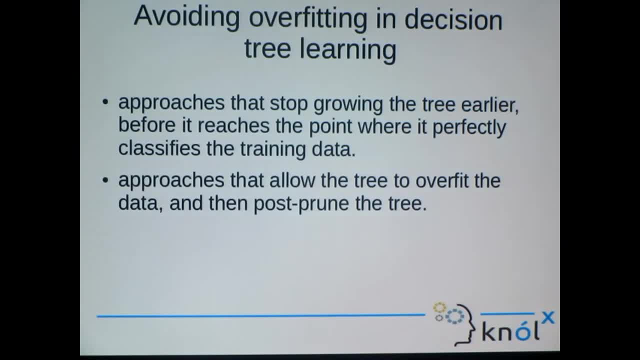 Prune means trim, As we trim the trees or grasses to give it a shape. We are going to do that thing here. Second approach is let the tree grow and then we will cut off the attributes which are not fine. So how to implement these two approaches? 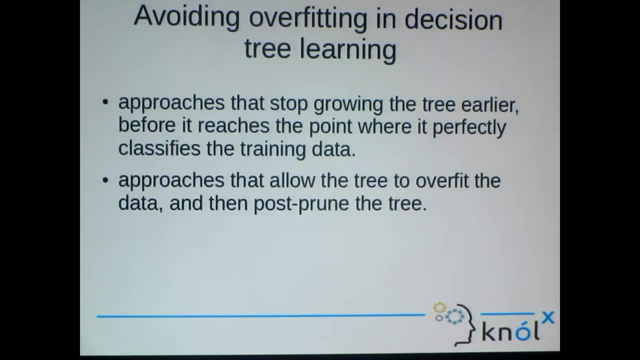 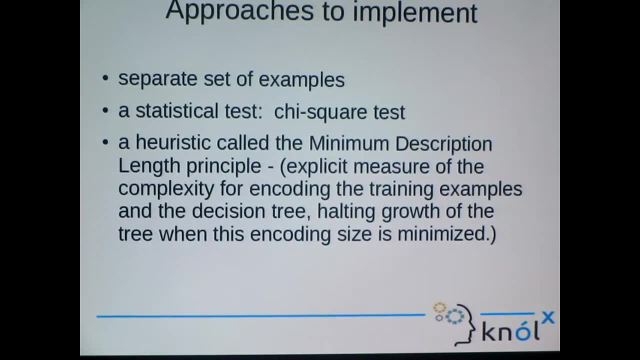 First is pre prune the decision tree. Second is post prune the decision tree. These are the approaches to implement. any of those approaches of over fitting, pruning First is separate set of examples. That means I have a data, huge data. 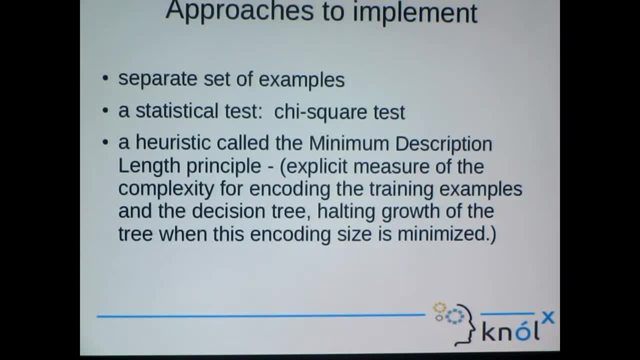 To build the decision tree, to test the decision tree. I am going to divide that big data with me into two categories: First with the training examples and second with the validation examples. Training examples will be used to build the decision tree and validation examples. 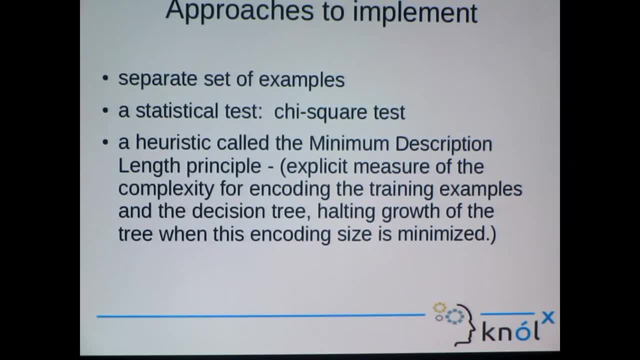 will help me to check whether my decision tree is correct or not. This is the first approach to implement pruning. Second is statistical test. Let us just use all the data with me as a training example, and then I will use some statistical test over it. 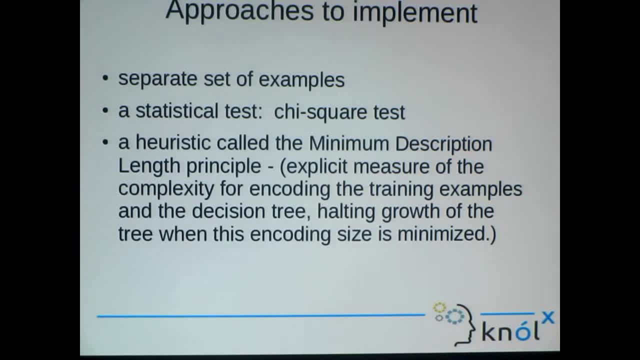 to check whether to prune or over fit the attributes over there. And third, one is minimum description. Minimum description, length principle, explicit measure of the complexity for encoding the training examples and halting the growth of the tree when the encoding size is minimized. I don't have much idea about. 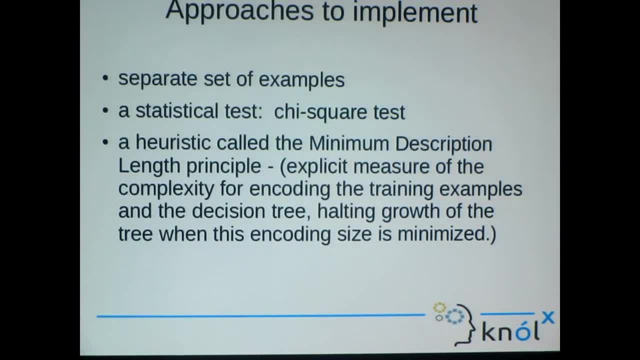 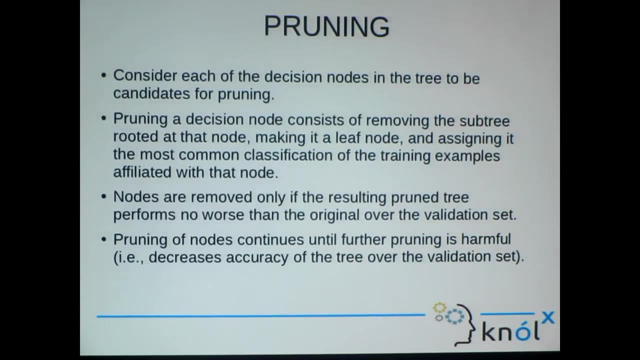 this last approach because it was not in my scope of the decision tree learning, So I am going to discuss first one more. So what is pruning? That is, I have made the tree. Now it ends up in a wrong decision tree. 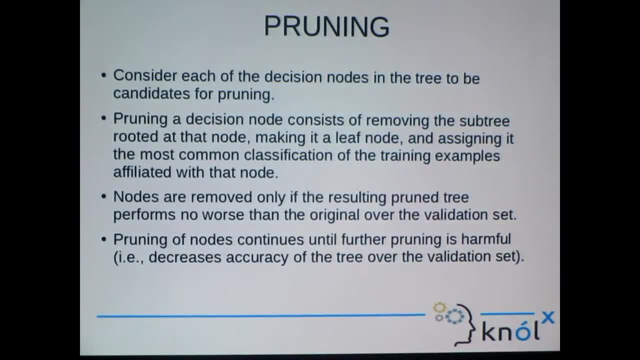 Now what to do. Pruning will help me in this. This is the whole process. Consider decision nodes in the tree to be candidate for pruning. each of the decision nodes, Every node, I am going to consider as my candidate for pruning. 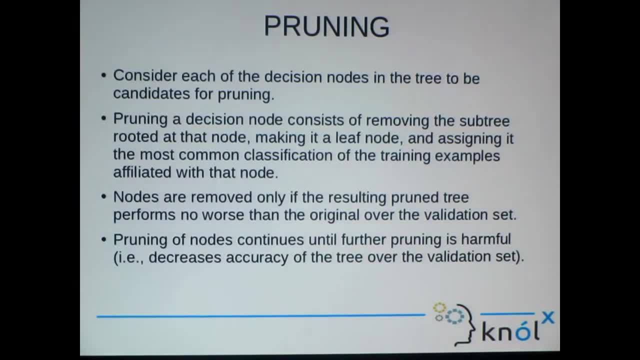 And now I will try and I will do. I will just remove the subtree of that particular node and check if it will affect the decision tree or not. Nodes are removed only if the resulting prune tree performs no worse than the original one. I will remove only that node. 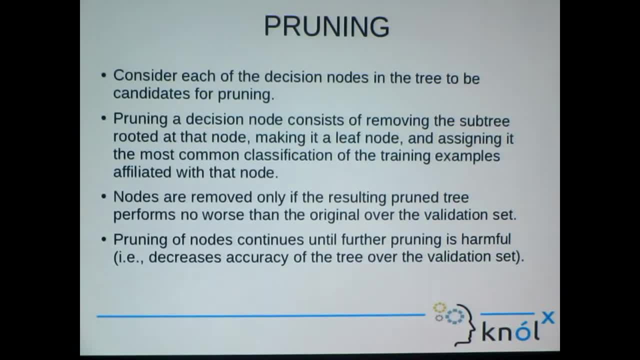 that will not affect my performance of the decision tree. It should either increase my performance or just remains the same, not worse than. And the pruning of nodes continues until further pruning is harmful. We are going to prune until it is harmful for the tree. 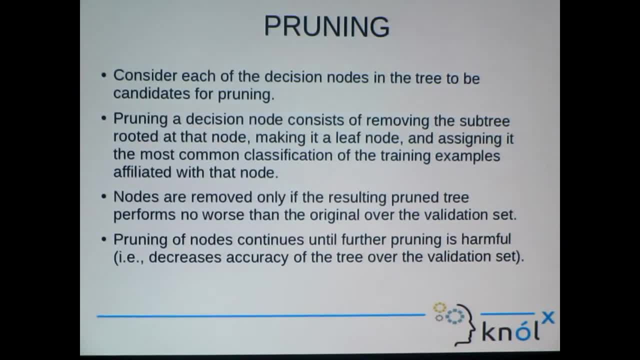 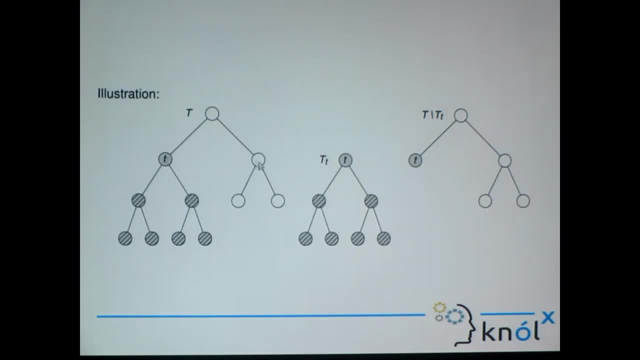 That means decreasing the accuracy of the tree over the validation set. Like this: This is a tree and I am going to consider each node as my candidate for pruning. So what I am going to do, I am going to cut this off, the subtree of that node. 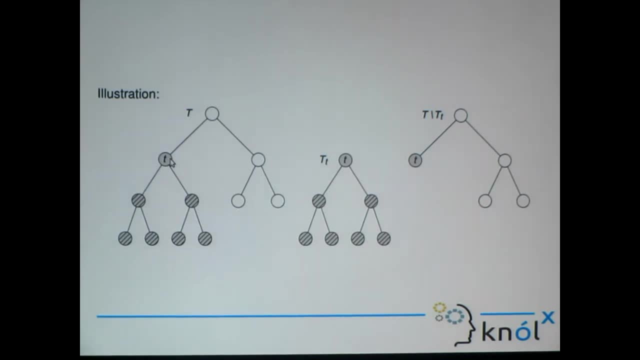 and make this T node as my leaf node And will check if it affects my performance of the decision tree. If it increases it, then it is fine, I am going to remove that subtree. If not, then I am not going to cut that off. I will go to some other. 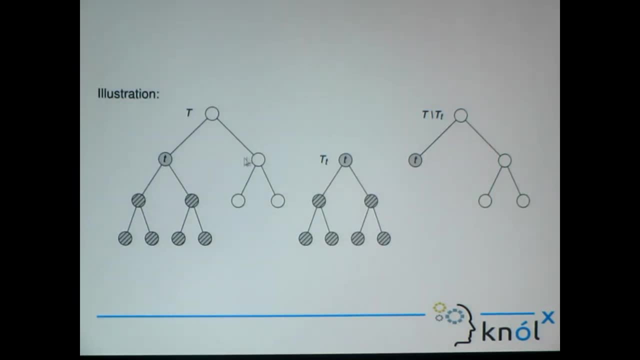 next attribute, next node for pruning process. Like this, It removes this one and make T as leaf node. Now, as a result, accuracy- this is the earlier graph. We have made the decision tree with my training, training examples- and accuracy is highest. 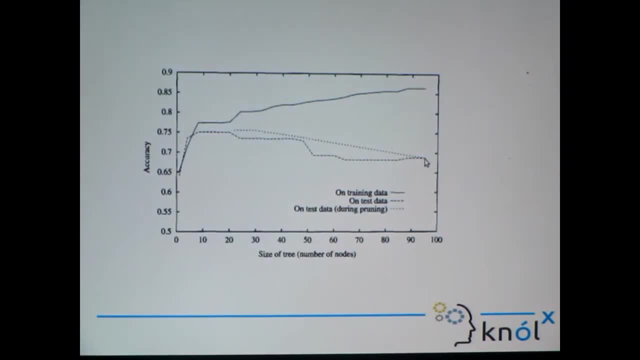 And when I check it with my validation set, it was not as accurate as the previous one. So this line represents pruning Right During pruning. This represents tree size When tree size is maximum. my accuracy is lowest When I prune the tree. 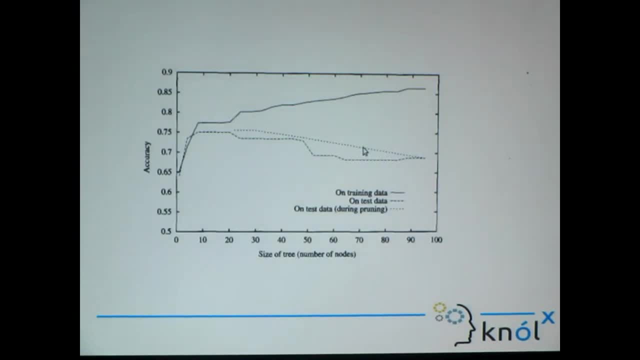 my accuracy. my tree size decreases and my accuracy increases, As you can all see. So pruning will help me- definitely going to help me- in decreasing the tree size and increasing the accuracy, But when we prune we have less attributes to check, Sorry, 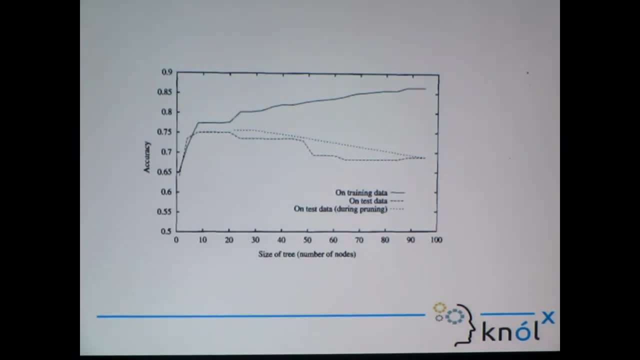 When we prune our tree, we have less attributes to verify our data, For example in case of animal kingdom, and when we prune the subset of the tree now, we have less attributes to check. So actually we are not dividing our kingdom in more fine categories. 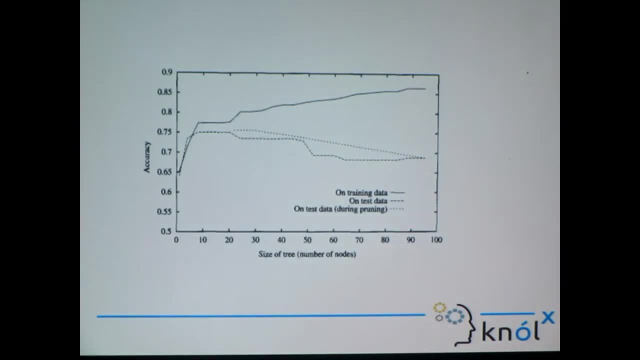 Now we have broader categories So the accuracy is low on pruning But it is not giving me good results Because now my categories those are more broad than before, But I need refined, fine categories. So I mean error rate increases, but it is not as much. 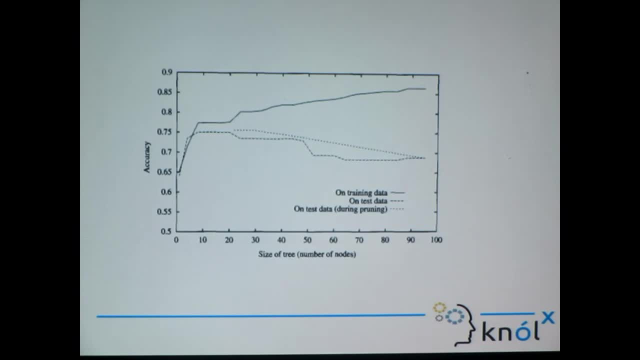 as good as it should be. Consider it not that good algorithm and we move to another algorithm. Basically, you decide between one of the two categories. So even after pruning I am getting better results, So it does not matter That four-legged attribute. 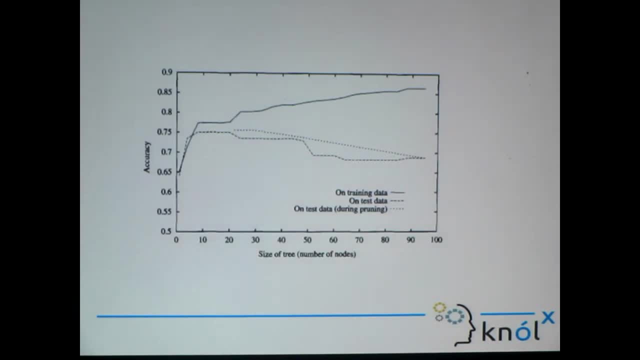 is not required at all. So why should I go to another node and decide whether it is a normal or not? Animals have two categories: Mammals, not mammals. But what if I want to further classify my mammals and non-mammals? 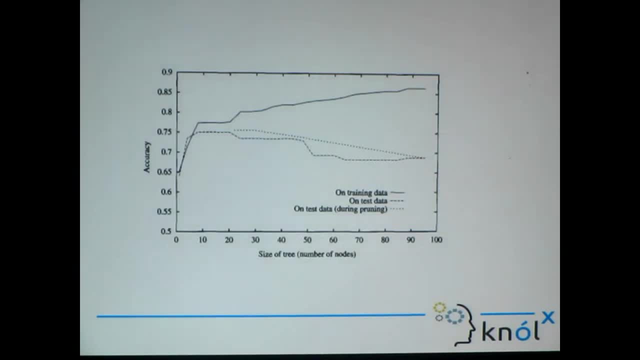 So but when I stop pruning, like I have so big tree, it can classify my animal kingdom. But if I prune it in just two categories, it is giving correct answer, The original intent of the decision tree, like the example Raman has shared. 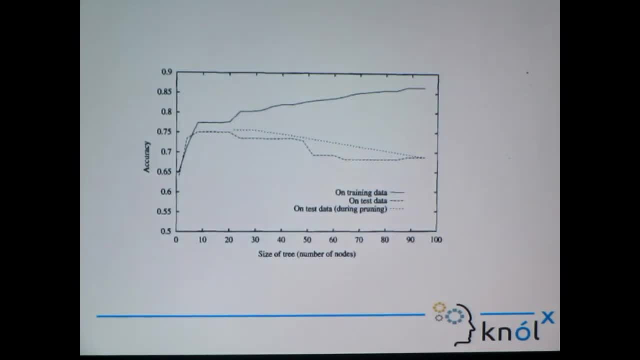 the intent of that decision tree is to decide between mammals or non-mammals. If you want to decide whether they are two-legged or two-legged, then you have to not consider the mammal. that is good. Then your order of the decision tree will change. 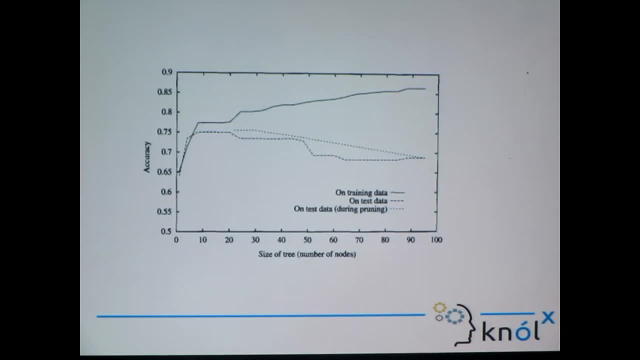 No, I am saying four-legged mammals. In that case error rate increases because mammals are not coming into that category. So if I prune it, then my categories decrease, But if I increase my categories error rate goes up. I guess my pruning helps you. 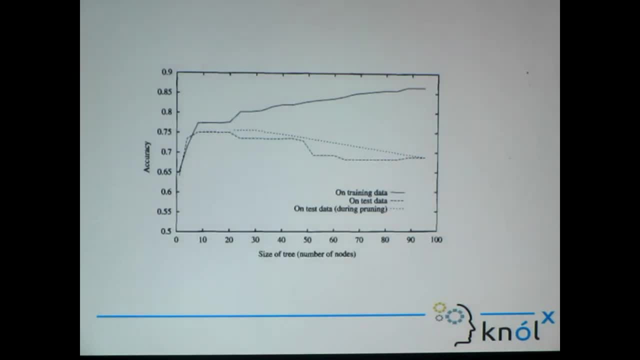 in removing bad data, right, And then you can retrain the data. No, actually we increase the training data set. Actually, when we prune the tree, then we increase the training data set. No, I am not saying to remove the bad data. 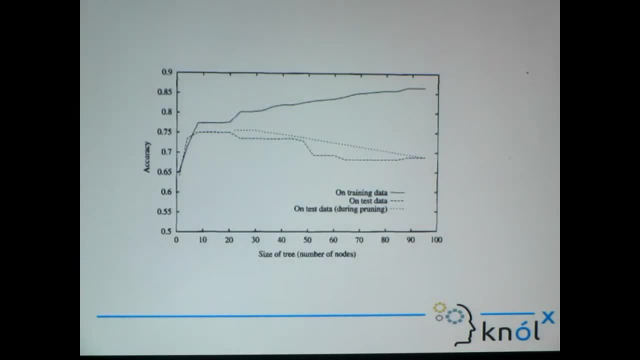 Actually, what happens is it was wrongly classifying the two-legged mammals for humans. The attitude itself is ambiguous. It is not ambiguous design. No. What Ashish is trying to say is we have categorized them into mammals and non-mammals. 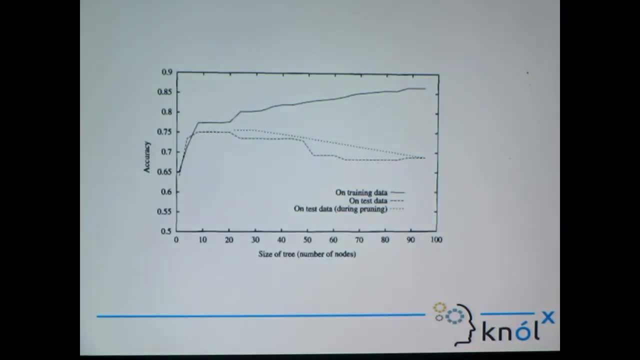 What if I want to know from my data whether it is a four-legged mammal or a two-legged mammal? That would be a altogether another situation. I mean, if I am saying that this is a different situation and this is different, then we are restricting. 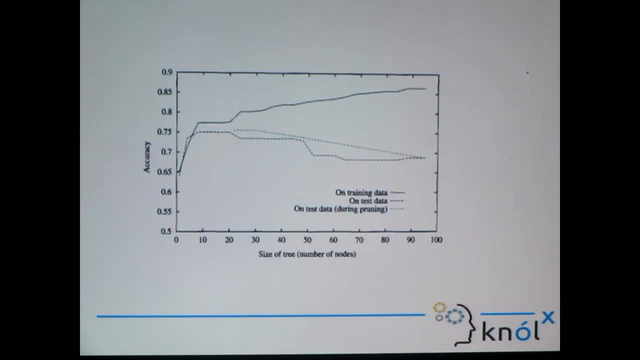 our machine It should be capable of, But two different decision would be made in that For that you have to use the render first. Just think about a machine which takes many samples and you can only give this set of commands to me. 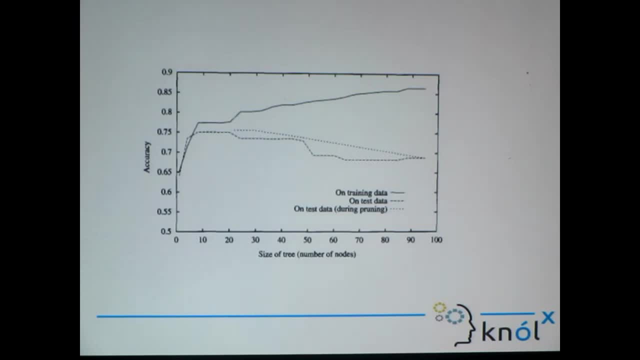 You are restricting your machine, But I want to make a machine which can. So, as he said, we are going to use random values and that is a collection of different decision trees. That is what I said last time, that we need to go to another algorithm. 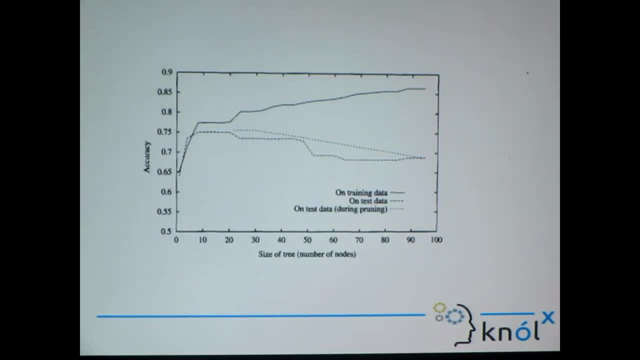 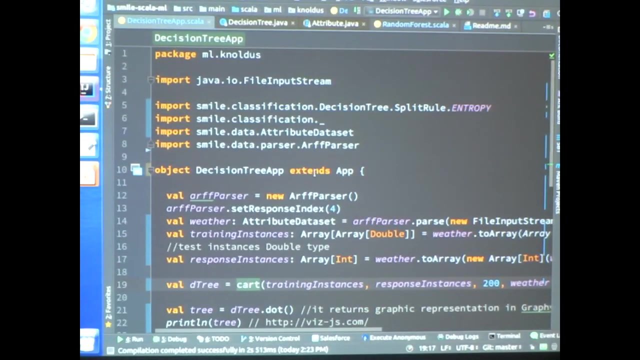 Not another algorithm, just a random algorithm. Then we can probably move on to the next one. How is this? Okay, Let me tell you about. Okay, I have used For this, I have used Smile Library for implementing decision trees. 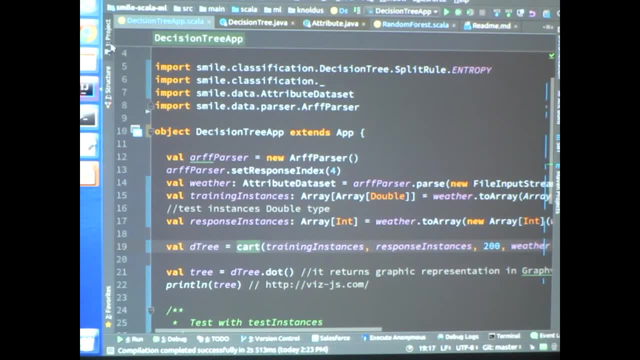 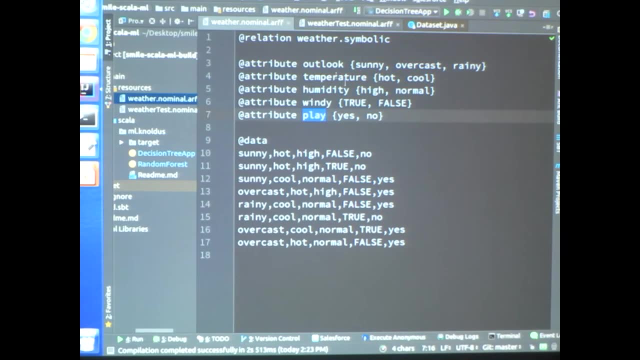 It will first start with the parcel I have given. Let me first show you the data. It is in ARL form. I have described the attributes- temperature, humidity, windy and play, and its values, like sunny, overcast, rainy and everything. 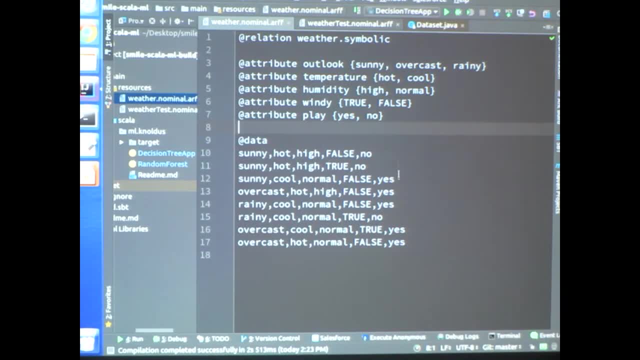 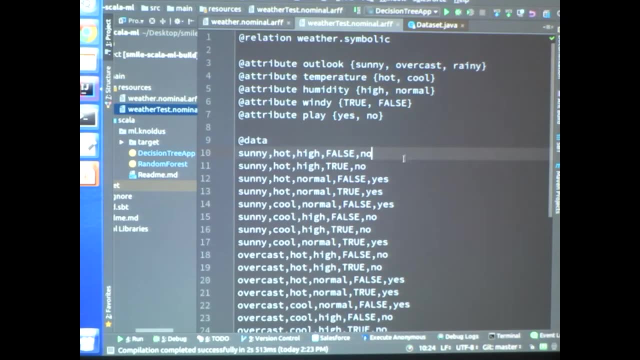 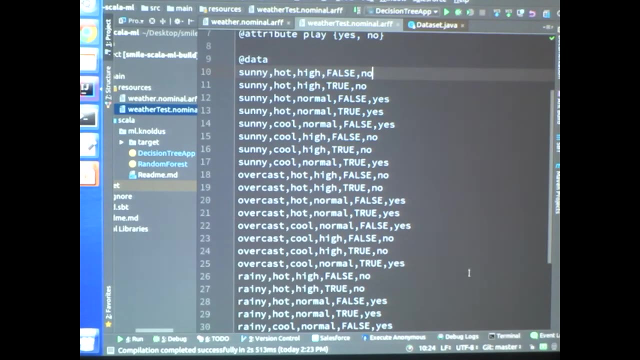 And this is the data. This is my training data. With this data, I am going to build my decision tree And, similarly, this is my validation or test data. I am going to check this data with my decision tree that I have made with the. 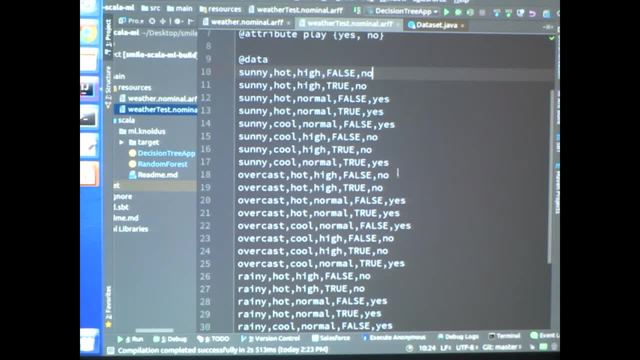 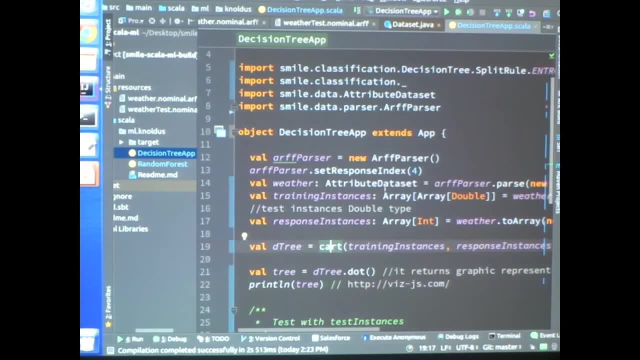 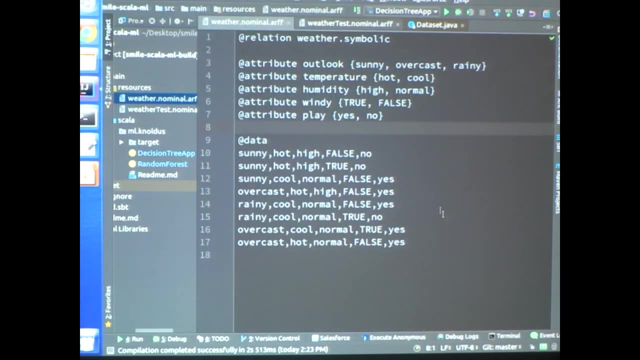 training set, And it contains some error data too, So it will give me error also. So first it will pass my data and I have set response index as 4.. And saying that my response attribute would be this: play, Play, whether, if. 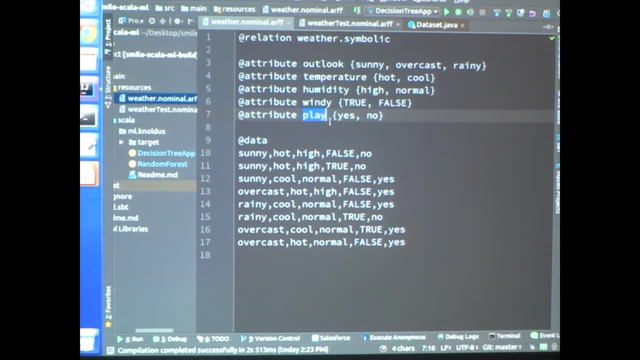 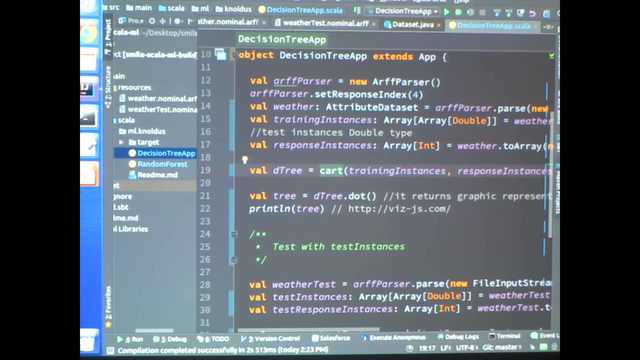 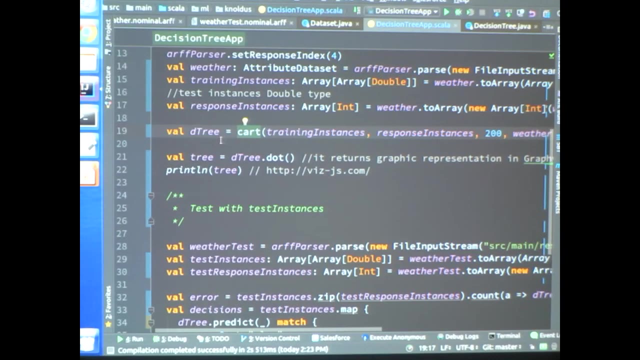 these attributes are in my favour, then I am only going to play outside. It will have values, yes or no. So the data is going to divide its training instances and response instances as arrays And this function card function, classification and regression trees. 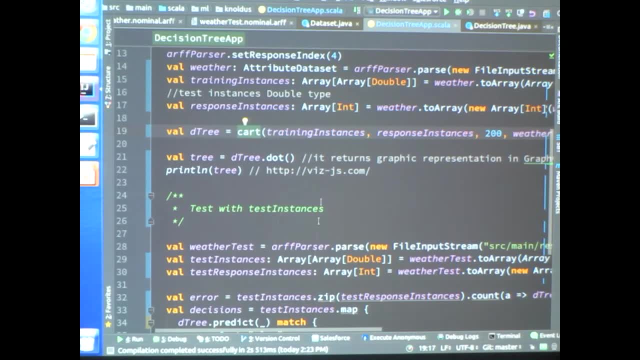 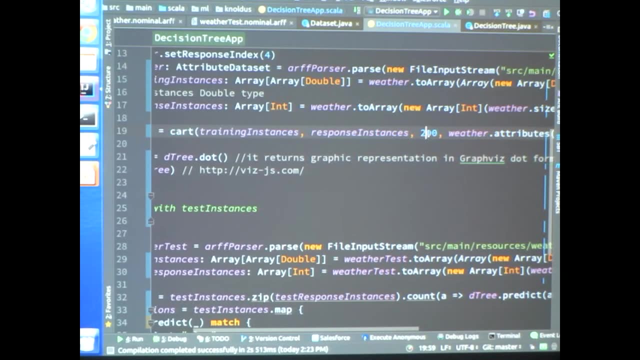 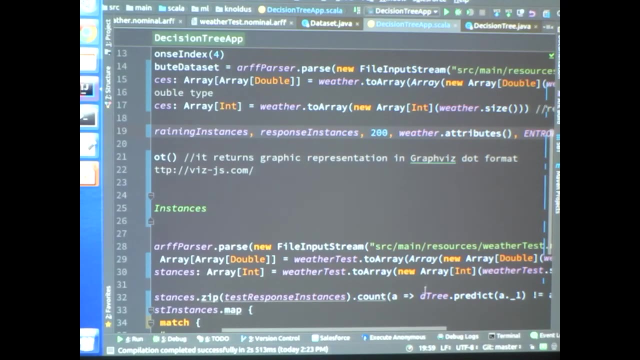 this is provided by SMILE and it is accepting the arguments like training instances, response instances and this is the maximum node length. I am going to give number of nodes and what are the attributes I am going to give? that is, outlook, all those things, And 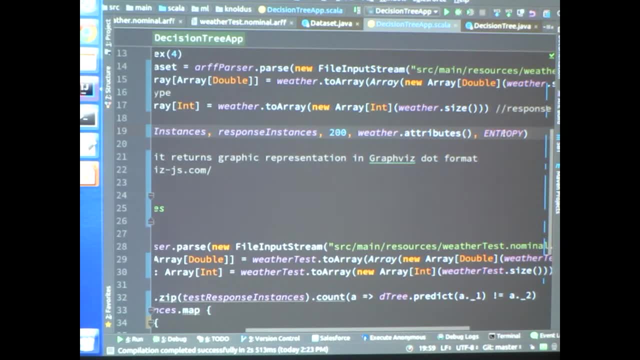 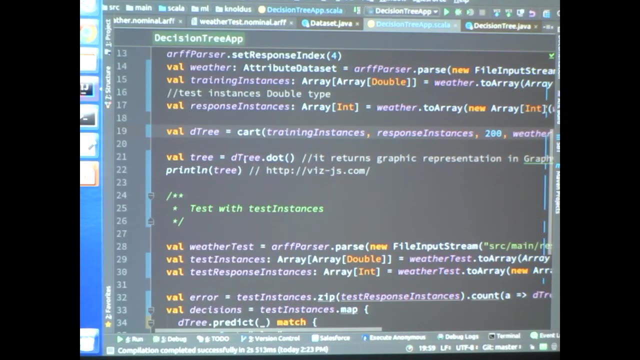 I am using which technique to implement that? that is entropy. There are also some other also techniques also like guinea and everything, And since I just taught you about entropy, So I am going to use entropy here, So this function will. 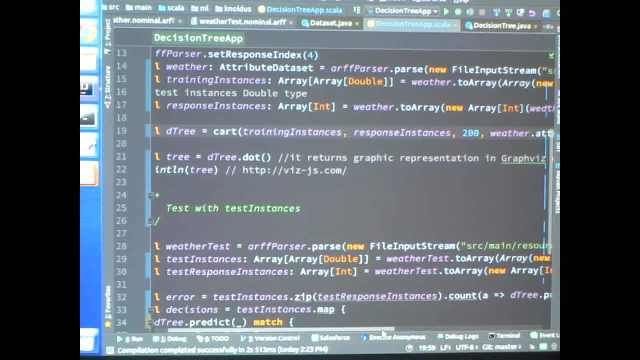 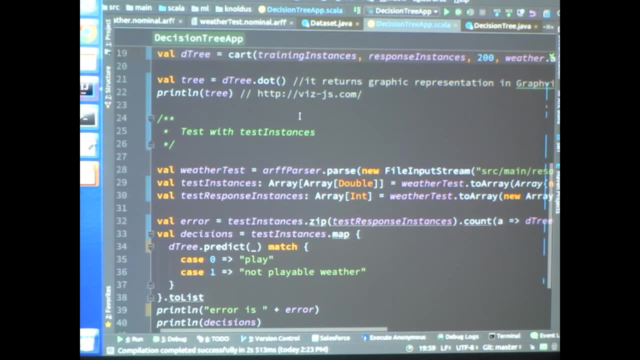 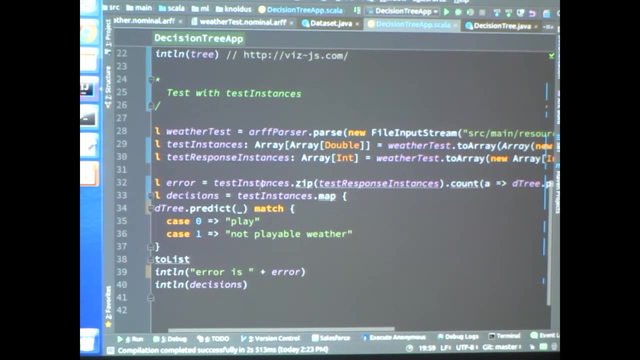 create the graphical representation of the tree And I am just printed. Now we are going to perform the same procedure for test instances And I am going to match See in there. here we are going to zip my test instances with my test response. 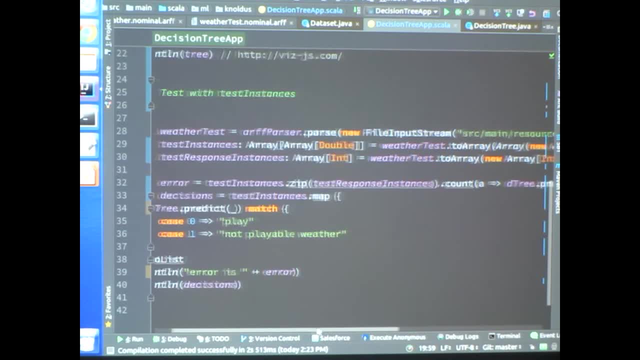 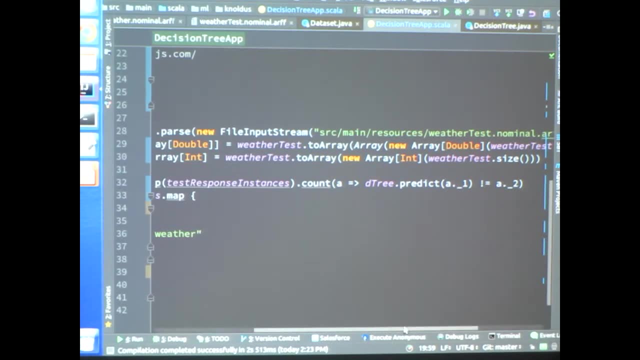 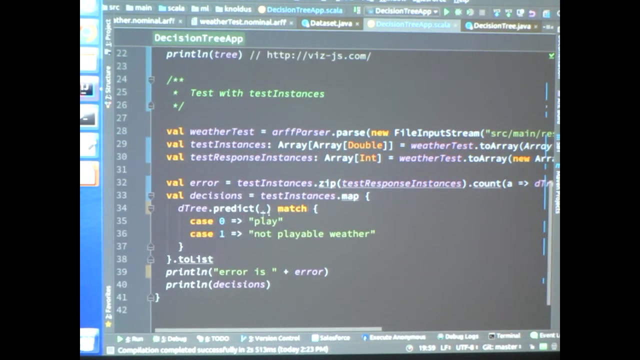 instances. Now we are going to count how many will predict the correct one and how many will not, And I am going to count which all records are not matching. So that will show my error And for the predicted ones, as it will get. 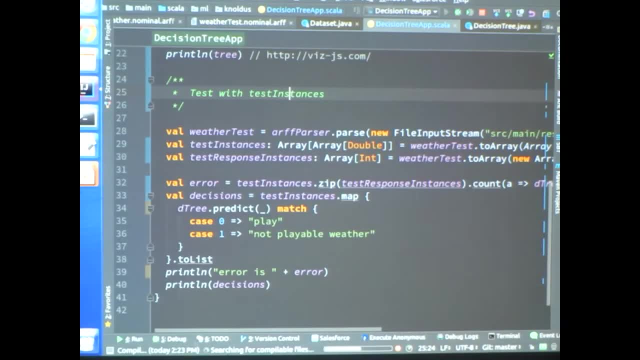 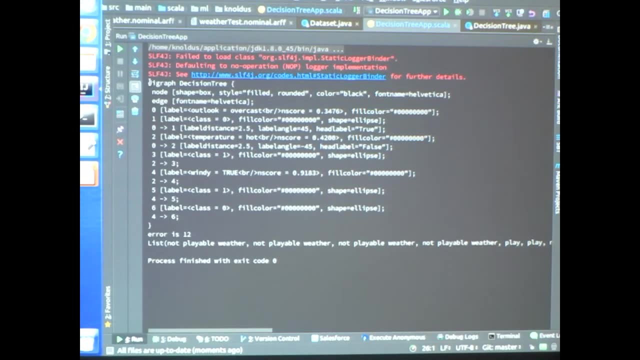 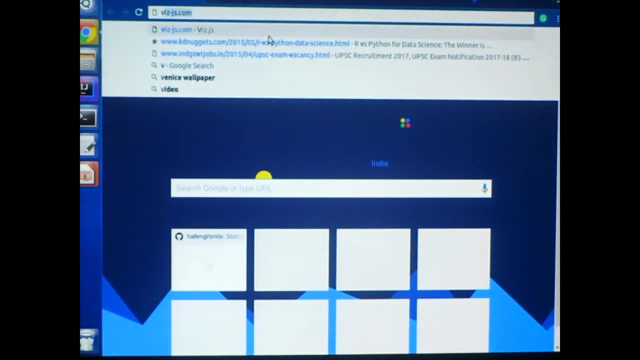 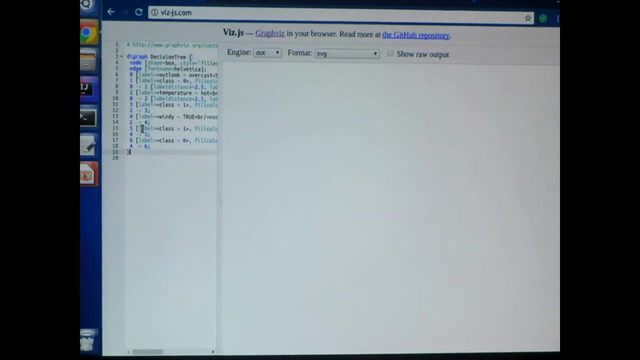 printed. So I am just going to run this one, So it will give me my tree in this form. And let me just show you this. This is the website. You can just put it. So it will. as you can see, my tree is. 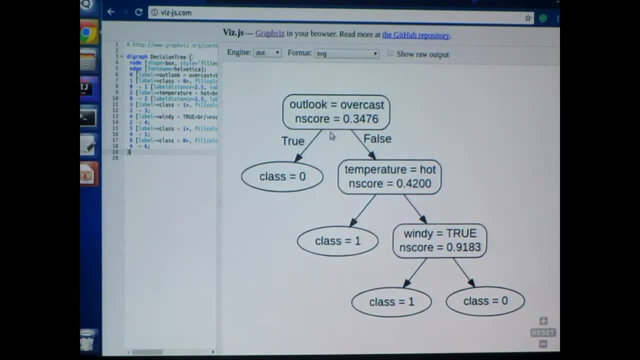 made with this outlook overcast. If it is overcast true, Then zero will present. yes, I am going to play outside, Right, And one will present. Okay, I am not going to play outside, So it will check our first. 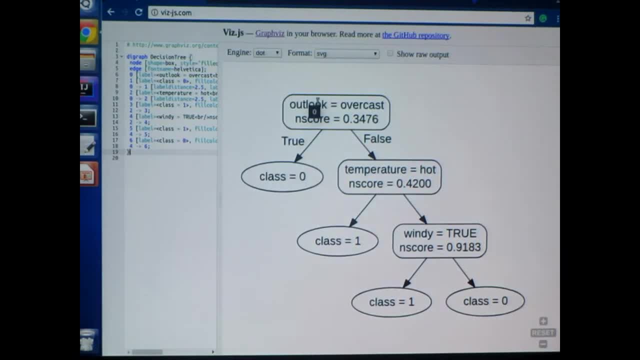 outlook. It selected outlook as its root node. So if it is overcast, yes, I am going to play outside. If it is not, then it will check the temperature. If it is hot, again, I am not going to play outside. 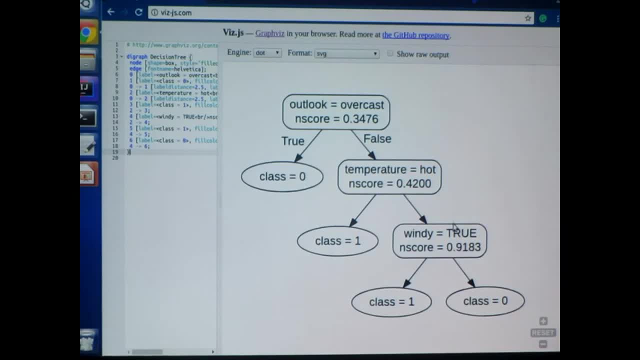 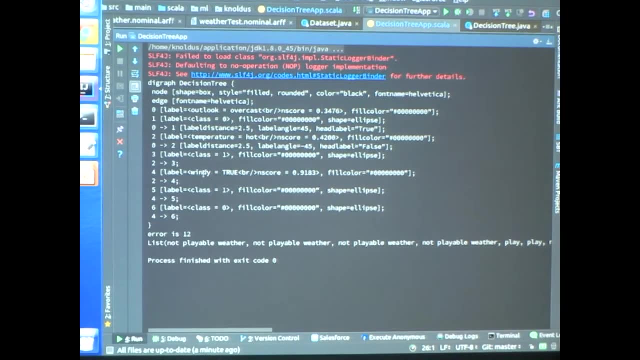 If it is not, I will check whether windy is there, whether it is windy or not, And the tree is made like that And, as you can see, error is 12, since I have given 12 wrong records in my training set over there. 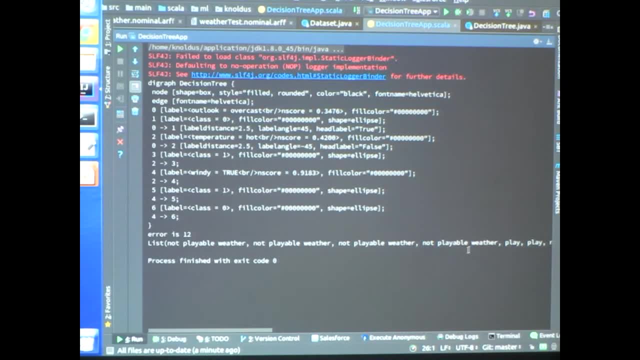 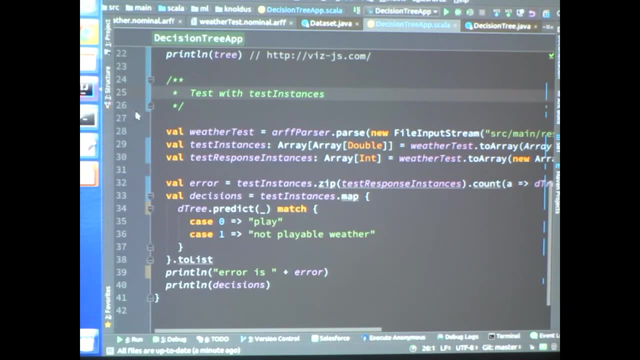 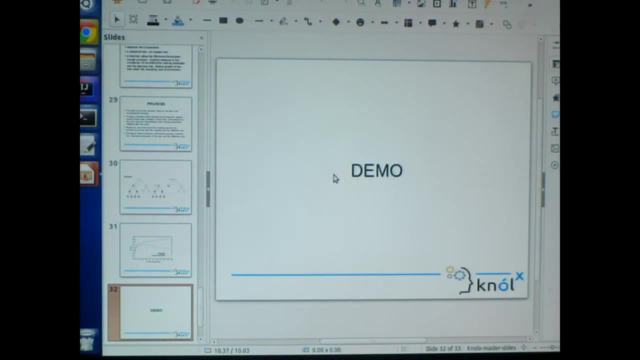 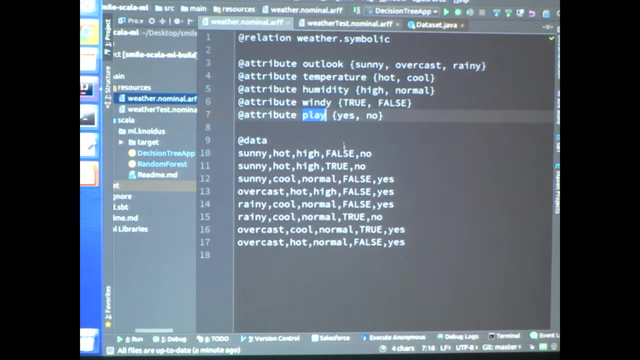 And it will print for all the active records, whether it can play or not. So that was all Any questions. Can we look at your training data? This is the training data, And decision tree is going to be based on this data only. 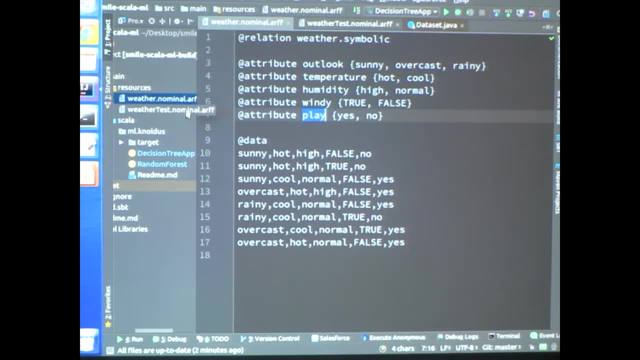 and these attributes. So this is also true, See, in decision tree. it is based on, as I told you, supervised learning, That we are providing it with the inputs and the desired outputs. also, This is the desired output, right And now.